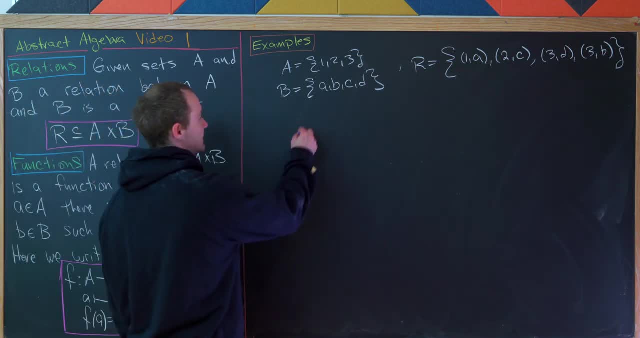 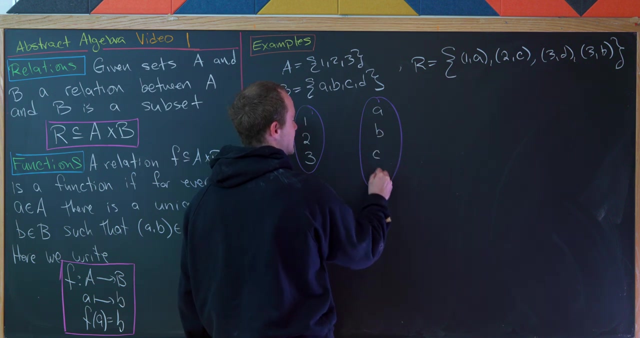 Now we could look at a graphical interpretation of this with like just a nice diagram. So let's say this is our set a. So it contains the elements 1, 2, 3. Let's say this bubble is the set b. So it contains a, b, c, and d. And then we'll simply put arrows between the elements 1, 2, 3, and the elements 1, 2, 3. And then we'll simply put arrows between the elements 1, 2, 3. And then we'll simply put arrows between the elements 1, 2, 3. And then we'll 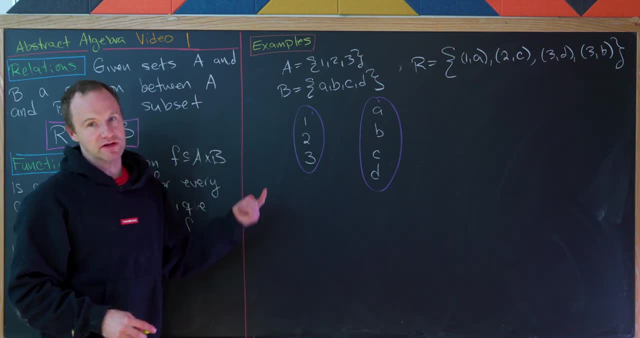 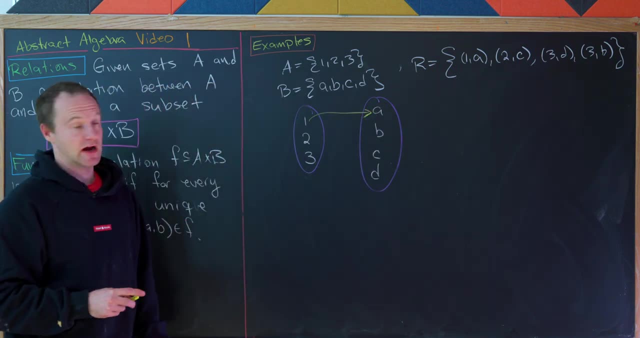 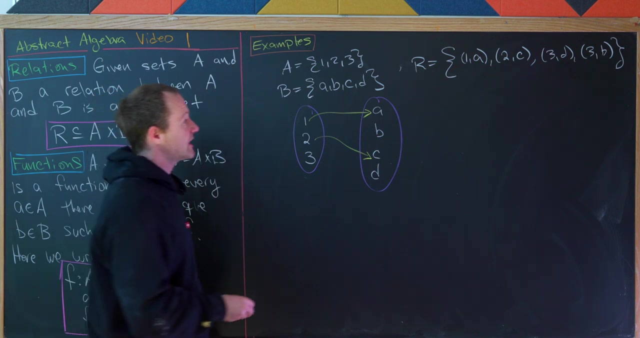 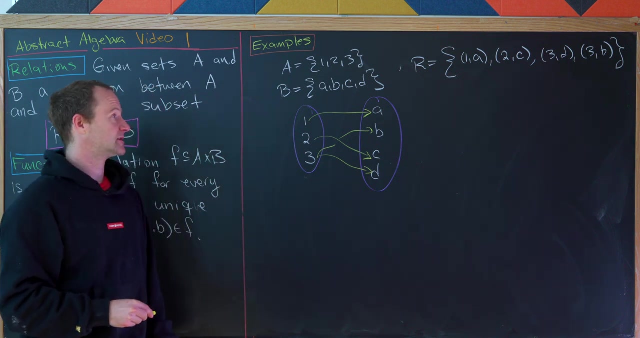 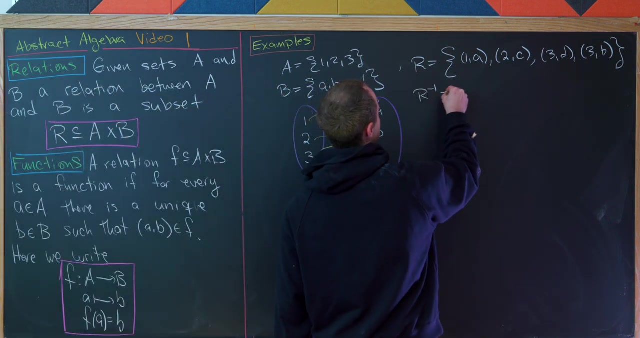 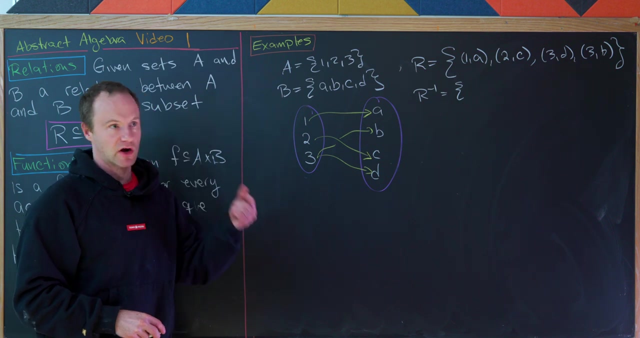 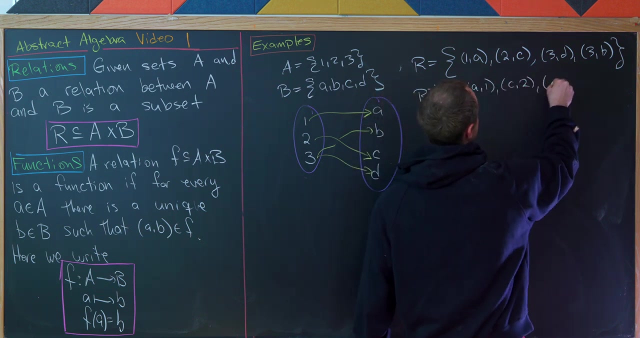 the elements from a that are essentially related to the elements in b. So that means 1 is related to a. We would write that as an arrow going in that direction. 2 is related to c. There's an arrow going in that direction. 3 is related to both d and b. So 3 has two arrows emanating from it like that. Okay. Well, there's also a notion of an inverse relation. And so we're going to So that would be simply the relation that we get from swapping the order of the ordered pairs. So instead of being a subset of a cross b, it'll be a subset of b cross a. And in this case, it'll contain a comma 1, c comma 2, d comma 3, and b comma 3. So I won't draw that, but that essentially 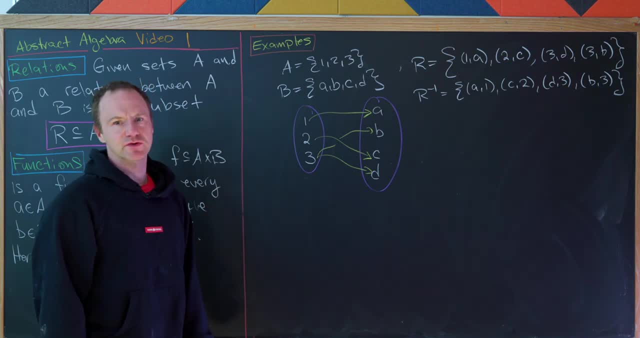 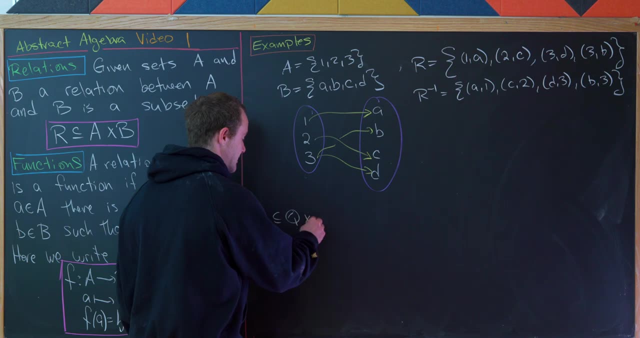 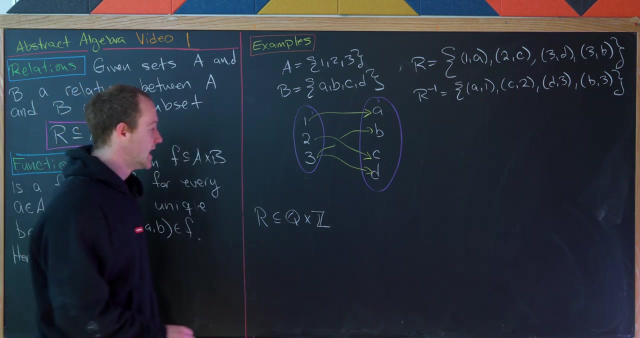 reverses the arrows. So I'd like to do another example. Let's consider the set r. So let's say r, which is a subset of the rational numbers cross the integers. So that means it's going to be a relation between rational numbers and integers. And what will it do? Well, let's say r 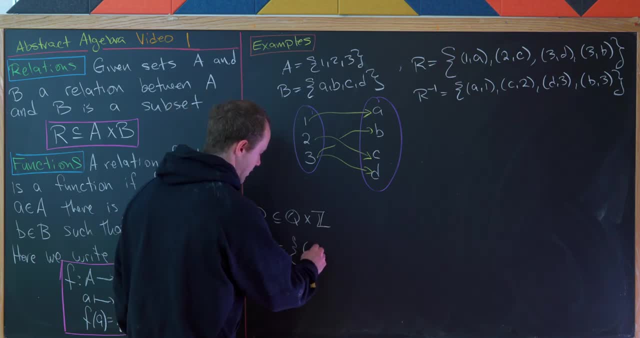 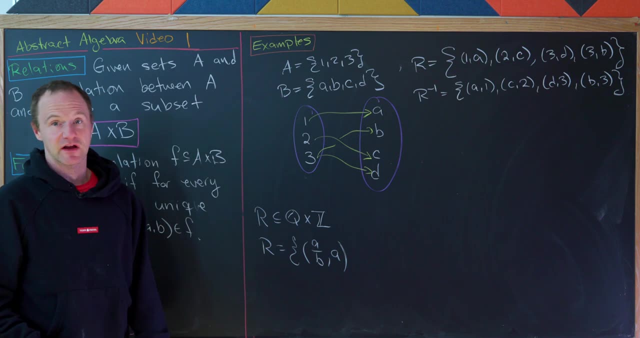 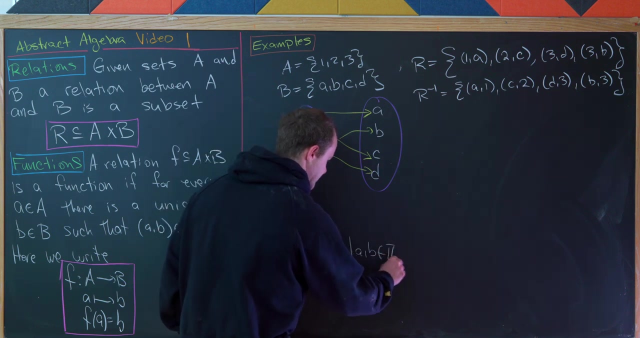 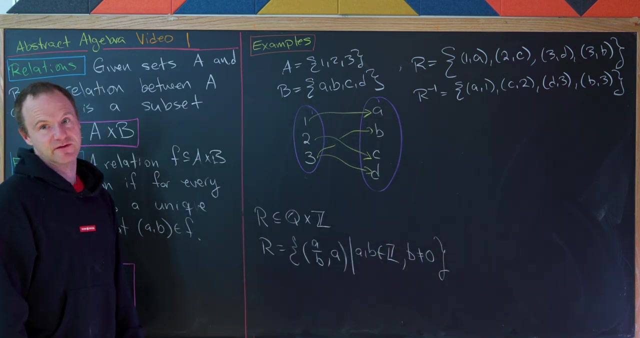 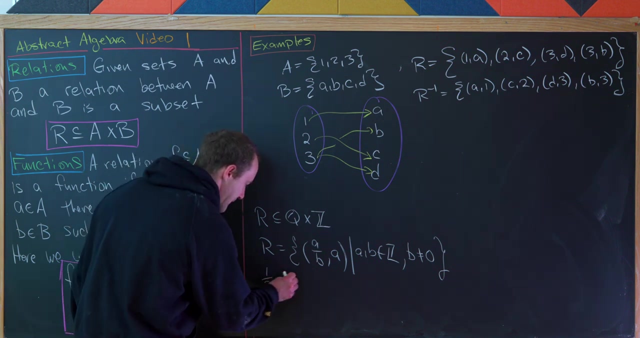 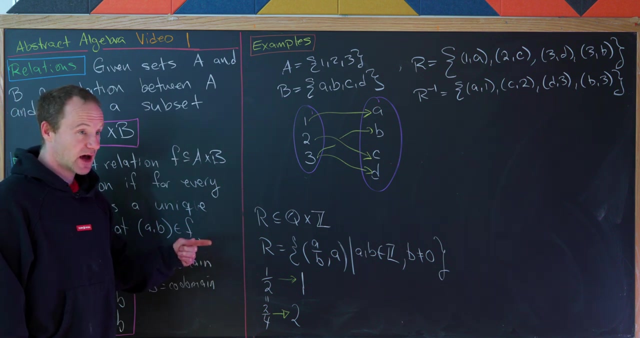 looks like this. Let's say it's of the form p over q, or maybe we'll use little a over little b comma a. So it's everything of that form. As a and b run through all integers, where b is not equal to 0. So that's most definitely an example of a subset of q cross z. So that makes it a relation between q and z, the rational numbers and the integers. So let's notice under this relation, we have things like 1 half would be mapped to 1, or would be related to 1 if we were to put this in this arrow notation. But now let's also notice that 1 half is the number of integers that we're going to be using. So we're going to have a the same thing as 2 over 4, but under this setup, we have that is also related to 2. So that means 1 half is related to 1, and 1 half is related to 2. Now, if alarm bells are going off in your brain, that's good, because you might be thinking that this is not a good way to define something. 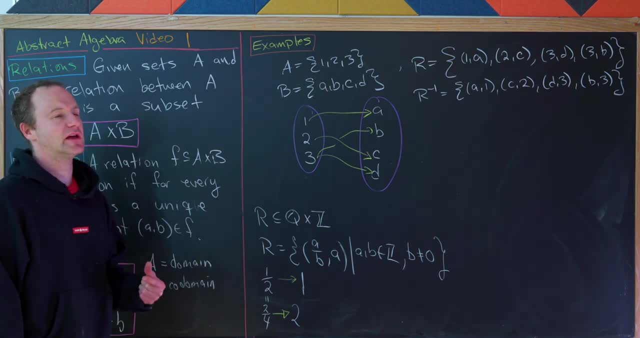 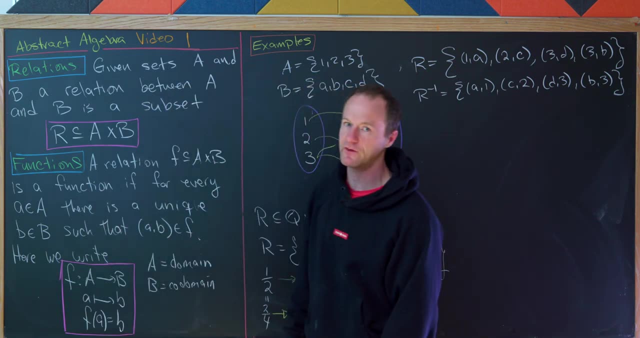 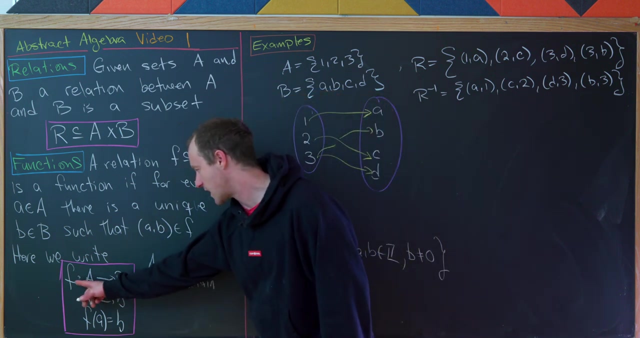 But this is fine for defining a relation, and what you might be thinking of is a function. And this, in fact, does not. It does not define a function. So let's recall the precise definition of a function in terms of a relation. So a relation f between a and b is a function if for every little a and a, there is a unique little b and b, such that the ordered pair a comma b is in f. So in other words, this little element of a is mapped to exactly one little b. And here we have like some standard functions, standard notation. So we might write f colon a arrow b. So that would be the setup that f is a function from a to b. Then you might say little a is mapped to little b under this function. We would use this notation. Notice we've got this little like starter vertical line to say maps to. 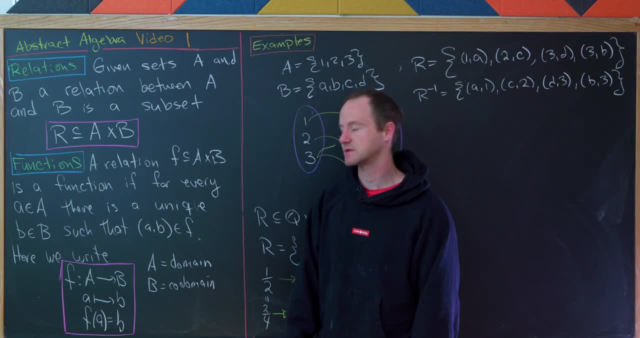 Or we might also say f of a equals b. That's more common in a calculus class. 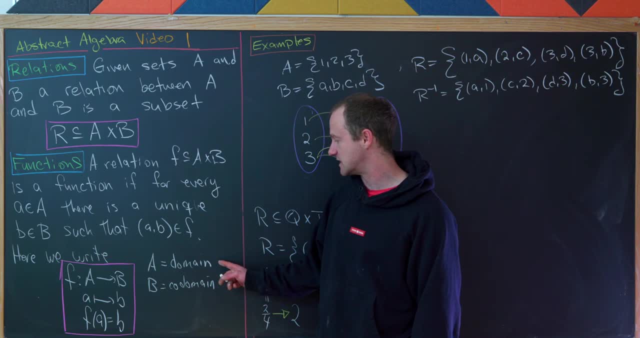 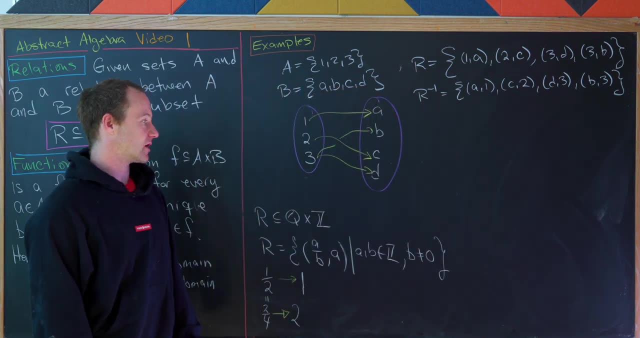 Then under this setup, the set a is known as the domain of f, and the set b is known as the domain of f. So we might write f of a equals b. And the set b is known as the codomain of f. So let's notice over here, neither of these are 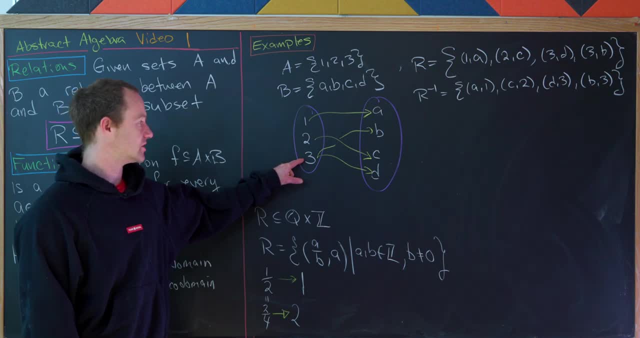 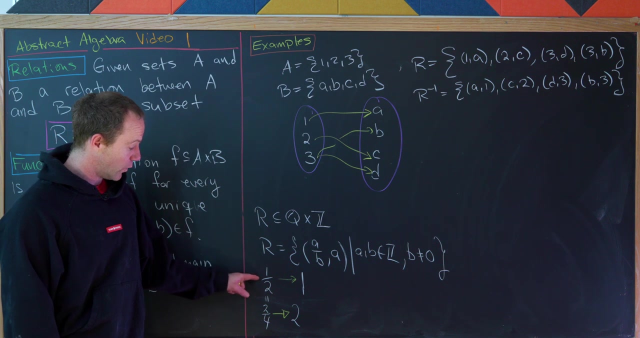 functions. So this first one is not a function because three is mapped to b and d. It is not mapped to a unique element of the codomain. And then down here, this one is also not a function because one half is mapped to one and two. Again, that's not a unique element of the codomain. 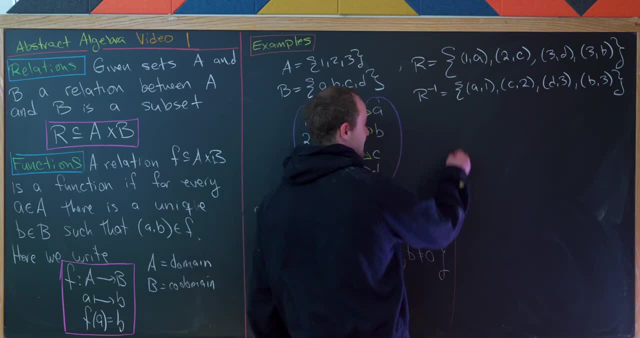 So maybe we could fix each of these to make them functions. And we could pretty easily. So let's maybe fix this first one. So let's say we have f going from a to b. And let's notice that 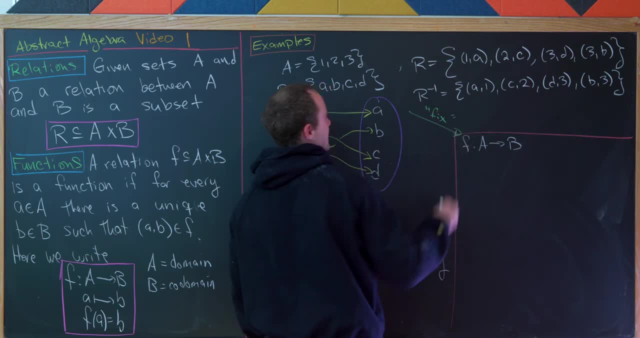 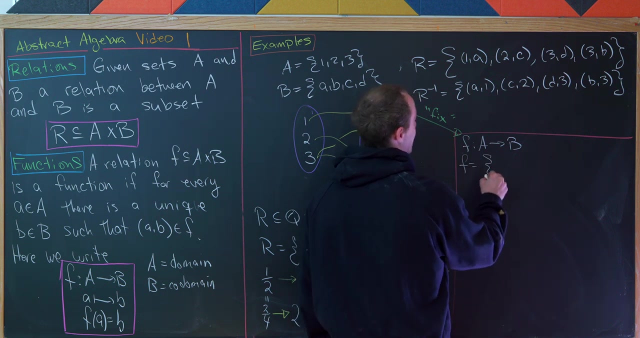 this is a fix. And what I mean is we're making it into a function. It's fine to have it like this and be a relation if our goal is not for it to be a function. And let's do that by maybe erasing the arrow between three and two. And then let's say we have f going from a to b. And let's notice that this isn't a function. So let's say we have f going from a to b. And let's say we have f going from and b. So in other words, now f would be the set of ordered pairs 1a, 2c, and 3d. And that would 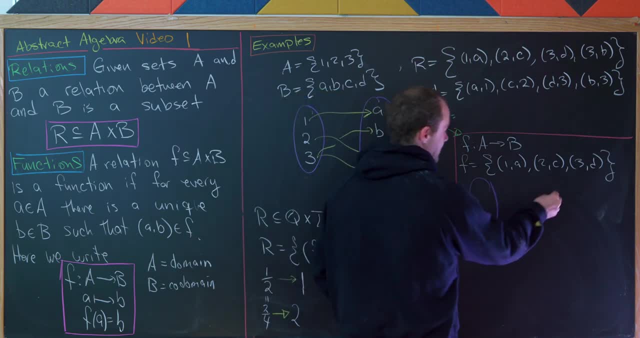 be totally fine. And like I said in this setup, what we've done is essentially erased the element 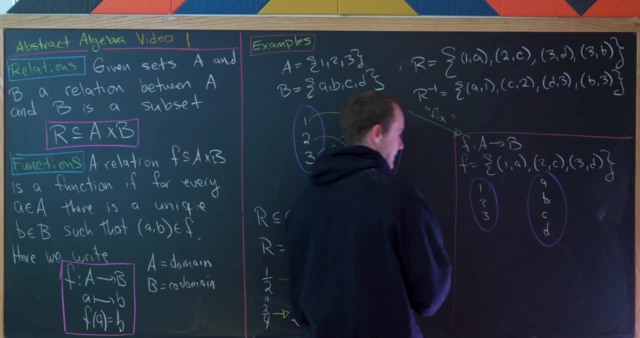 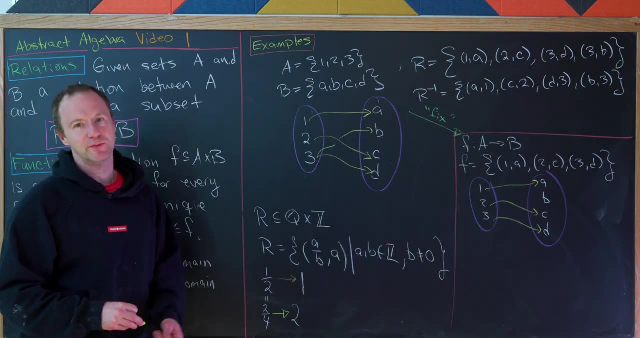 from 3 to b. So we're left with something like this. One is mapped to a, two is mapped to c, and three is mapped to b. Notice that b is not mapped onto by a and three and d, but instead by a and a plus. Notice that you notice our sign is now on midpoint one over two, and this why amigos might have different order pairs and take away our $10 or twenty thousand. So in this logic, we're saying r equals 30. If that would be the Biermannเหpsch in our idea of ordering a million is not mapped onto by anything but that's totally okay. And then you might say well how could we fix 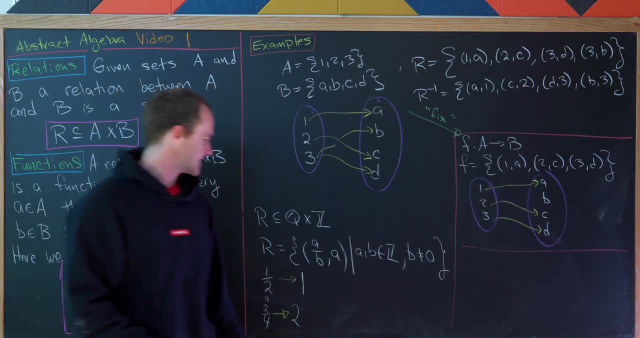 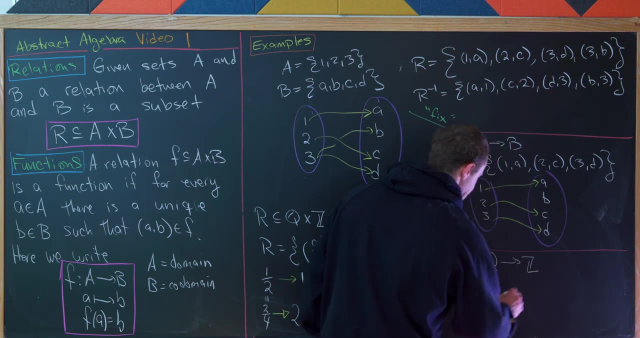 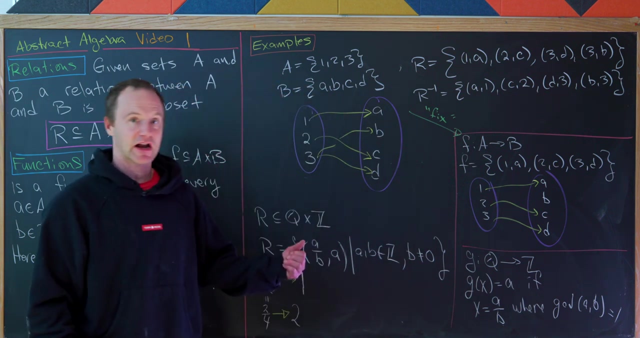 this second setup? Well maybe we'll fix it like this. Maybe we'll say that that g is a function from q to z and we have g of x equals a if x equals a over b where the gcd of a and b is equal to one. That means that our fraction is in lowest terms but if our fraction is in lowest terms then that means the numerator is unique but that makes that means we have a unique assignment 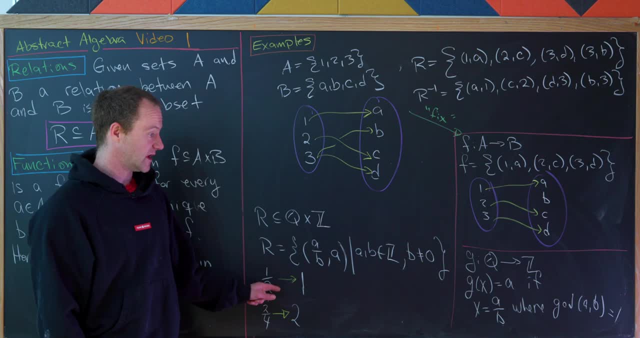 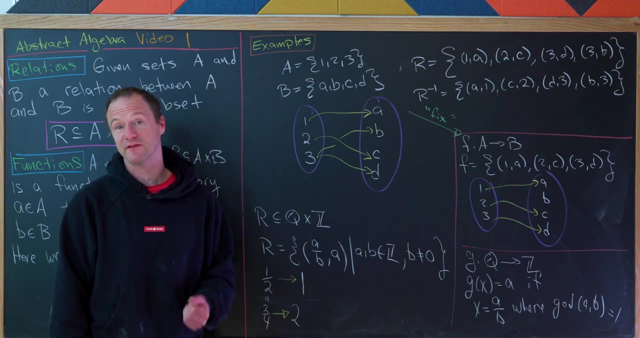 here. So that'll make this kind of awkward thing here into a function. Okay so now that we've reviewed relations and functions I'd like to look at some properties that functions can have. So let's recall the following definition. So let's say we've got a function from a to b where we've got a function from a to b where we've got a function from a to b where we've got a 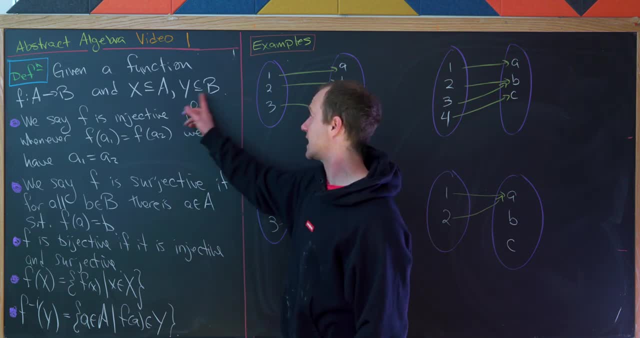 we have x is a subset of the domain and y is a subset of the codomain. So first we'll say that 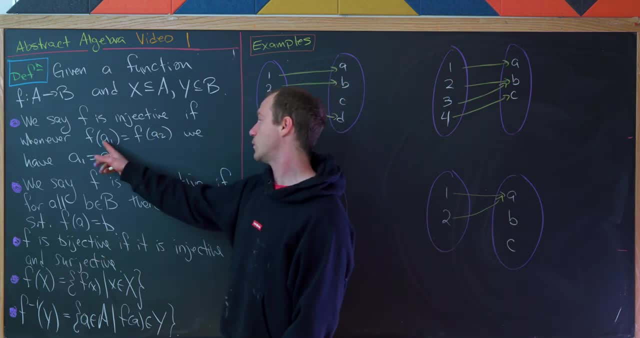 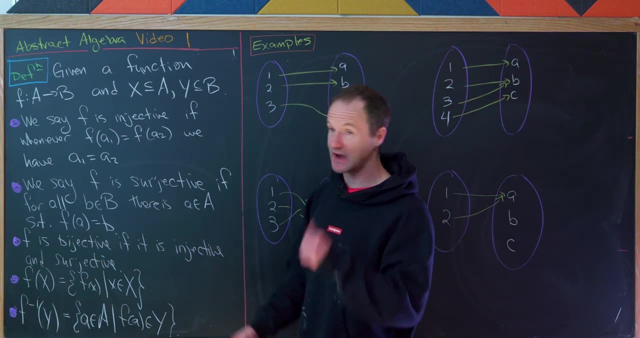 f is injective or one-to-one if whenever f of a1 equals f of a2 we have a1 equals a2. Then we say that f is surjective or onto if for all b and b there is an a and a such that f of a equals b. Then we say it's bijective if it is both 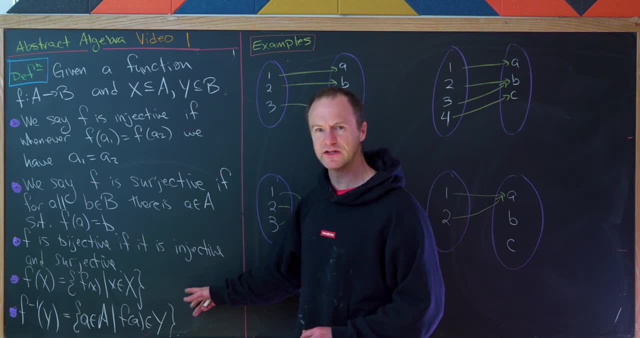 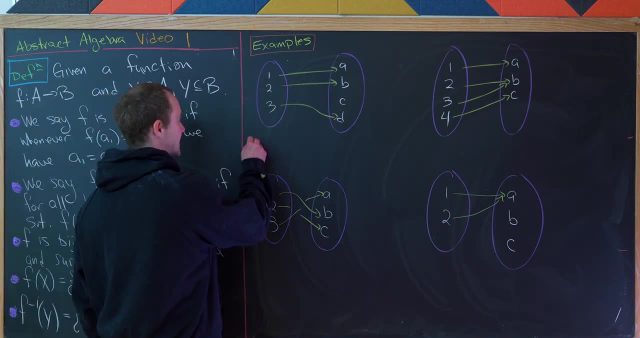 injective and on to. So let's say that f is surjective or onto if for all b and b there is an injective and surjective and then we'll cover these in just a second. So let's look at the following examples. So let's notice that this first one is injective but not surjective and 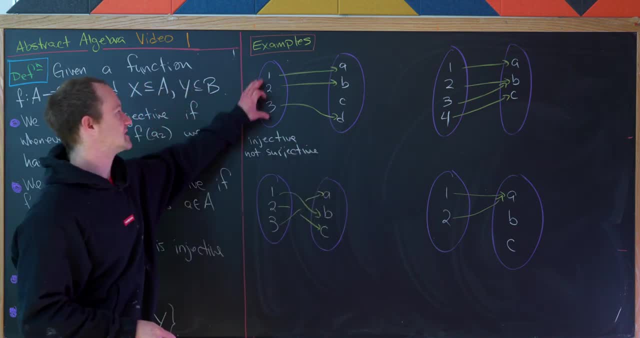 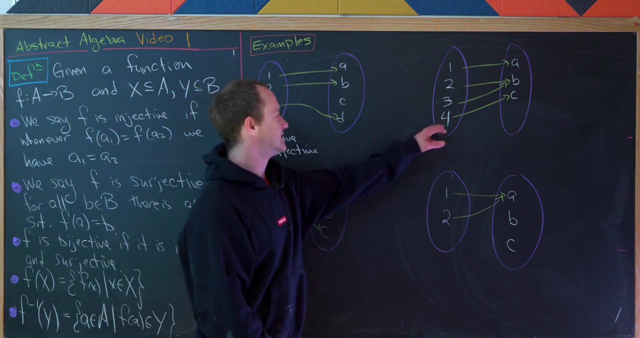 that's because no two elements of the domain are mapped to the same element of the codomain. They're all mapped to different elements of the codomain. It is not surjective because this element c of the codomain is missed. Now let's look at this next one. So this one is surjective. That's because 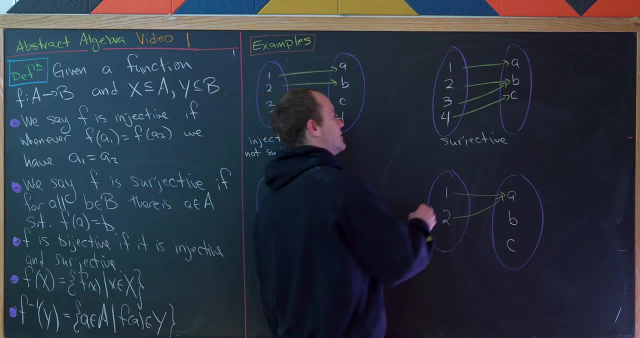 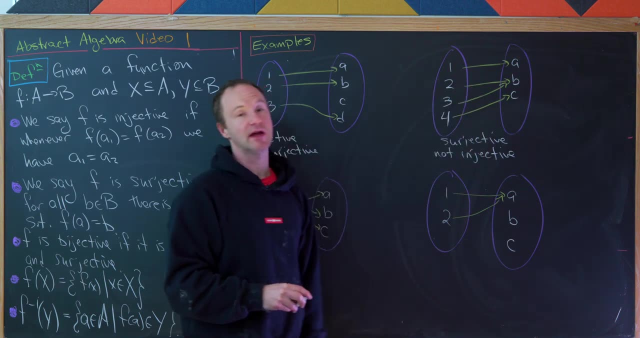 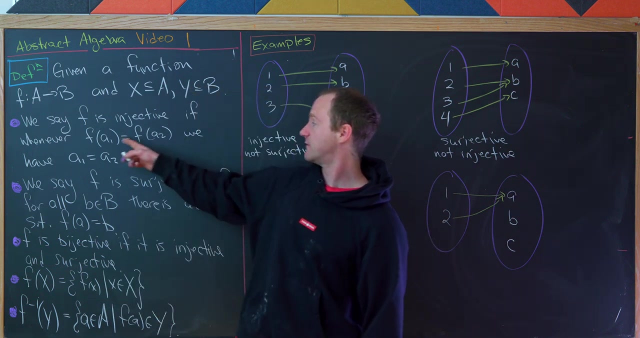 everything in the codomain is landed on by the function but it is not injective. And we see that it's not injective because two and three are both mapped to the same element of the codomain. So that means it doesn't satisfy this rule right here. f of two equals f of three but two is not equal to three. 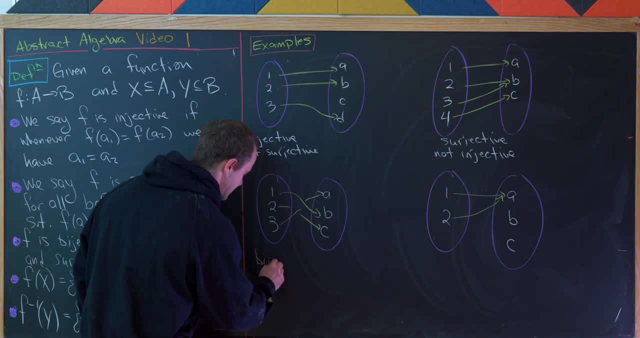 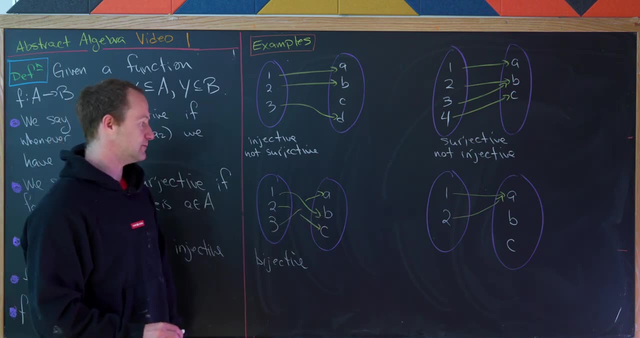 Now let's notice this one right here is bijective and that's because well it satisfies injectivity and surjectivity kind of clearly. One is mapped to b and only b. Two is mapped to c. Three is mapped to a. So everything in the codomain is landed on and it's only landed on by one element. 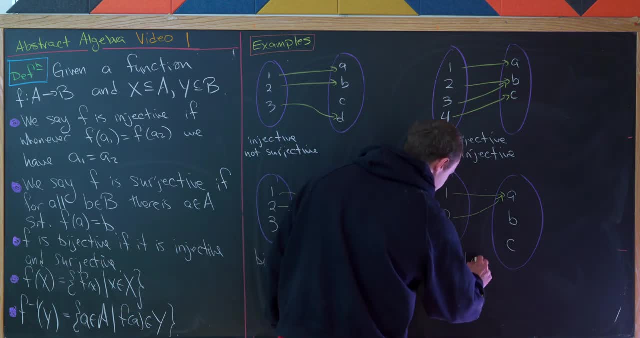 Now let's notice this one over here is neither injective nor surjective. Okay so now let's look at the second part of our definition and that is the notion of image and preimage. And that's going to require these subsets of the domain and codomain. So the image of a subset of the domain which we'll call f of x that's capital x. So that's going to be everything of 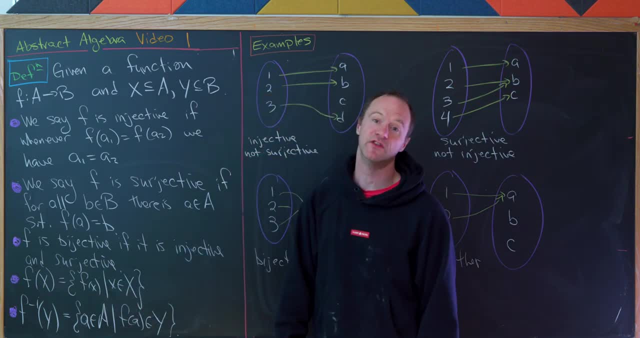 the form f of little x as x runs through all of the elements of capital x. And then the preimage which we'll say f inverse y or the preimage of y 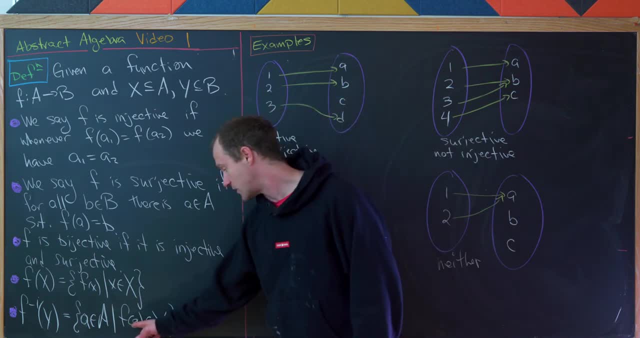 will be all elements of the domain so that those elements of the domain are mapped into that set a. So let's notice that the image of a subset is inside of the codomain whereas the preimage 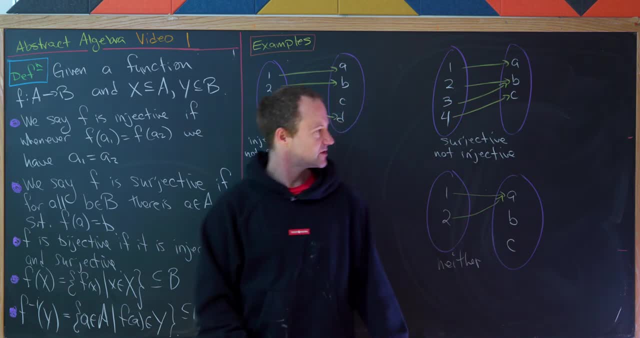 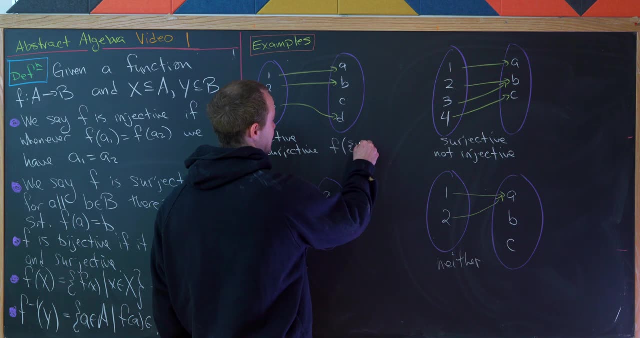 is a subset of the domain. Okay so let's look at some examples over here. So in this case let's maybe look at the image of the set containing one and two. 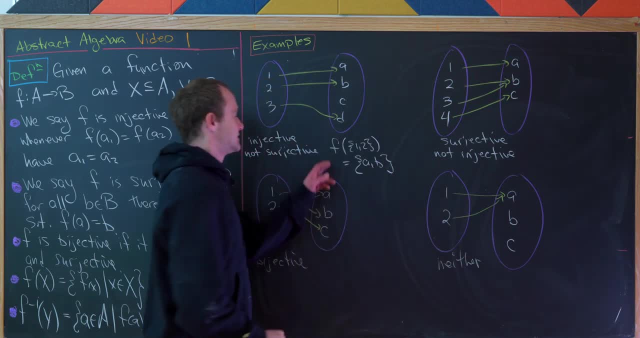 So that's going to be the set containing a and b. It's because f of one is a and f of two is b. 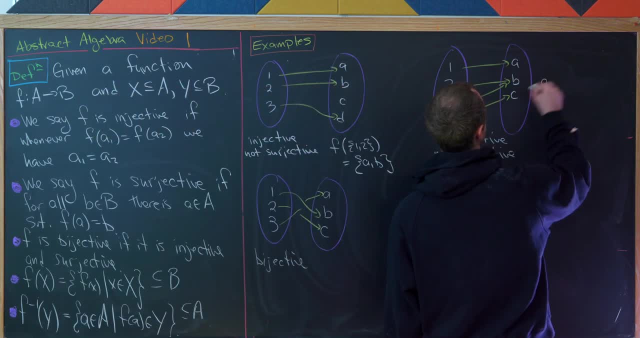 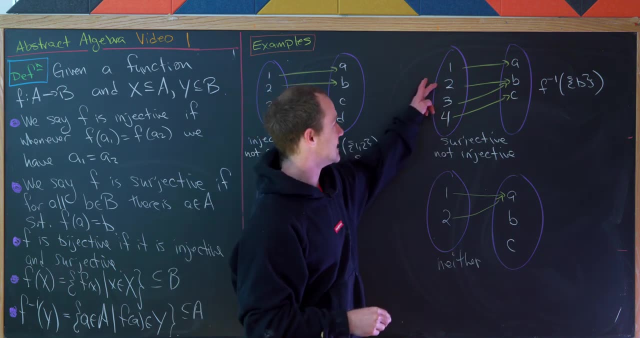 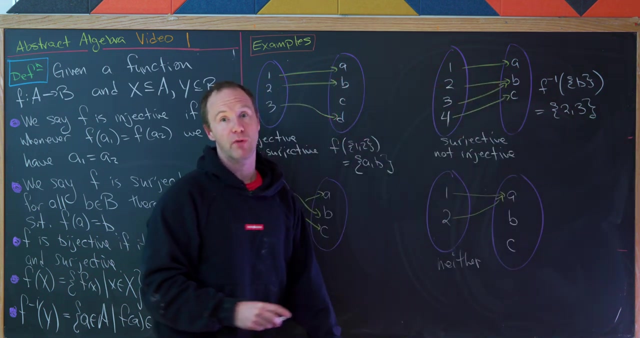 Now let's go over here. Let's look at maybe the preimage of the set containing b. We'll notice the preimage of the set containing b will be the set containing two as well as three. That's because two and three are both mapped onto b. Let's look at the image 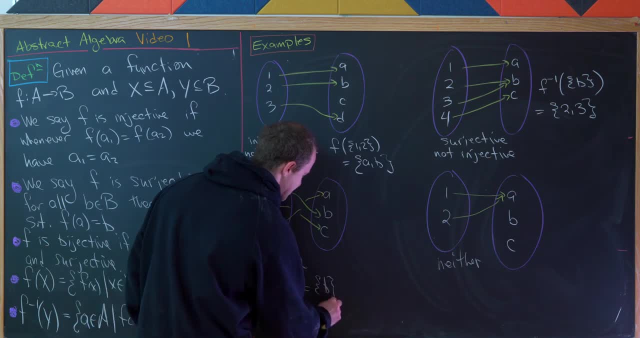 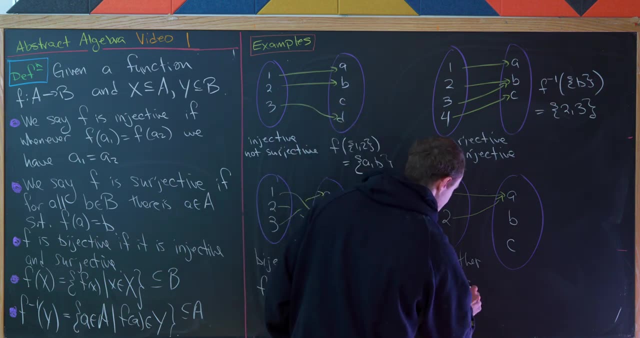 idea of the preimage of the set containing one. Not super interesting but that's going to give us the set containing b. Now over here let's do something interesting. Let's take the preimage 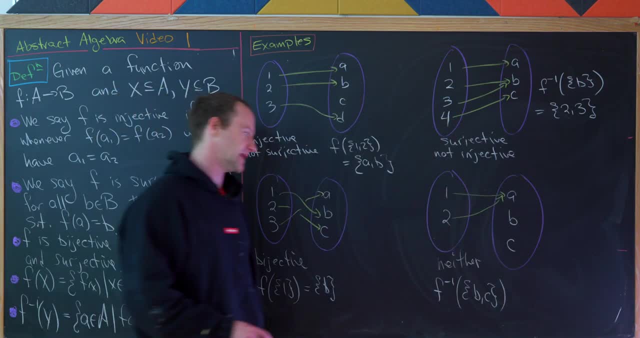 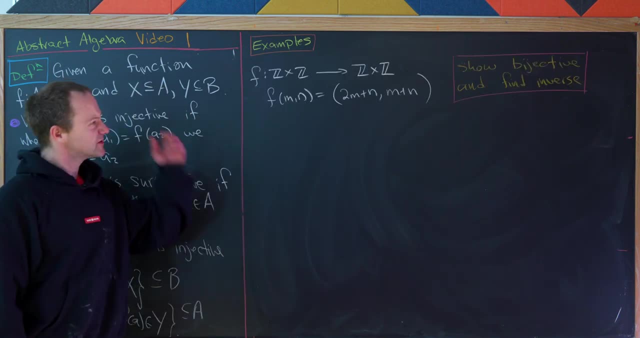 of the set containing b and c. But notice nothing maps on to b and c that makes this preimage the empty set. Now let's do some more calculation based examples. So let's look at the following example. We'll take f which goes from z cross z to z cross z. 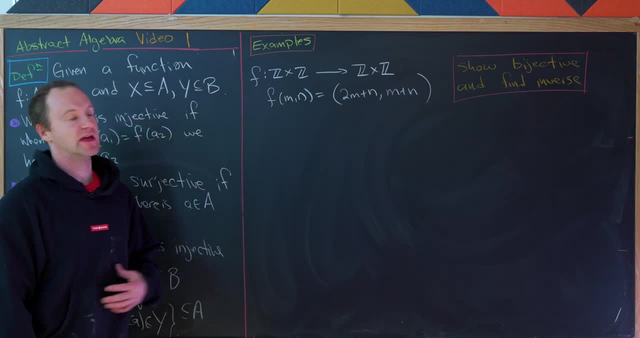 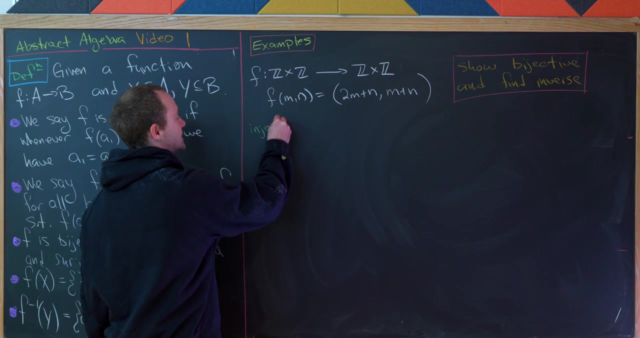 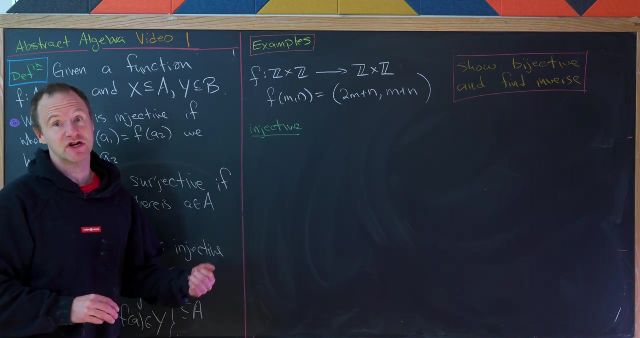 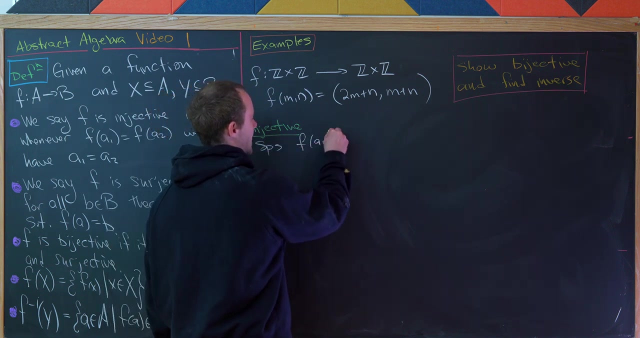 takes m comma n to 2m plus n comma m plus n. So let's recall that z cross z is going to be all ordered pairs where the first and the second entries are integers. So our goal is to show that this thing is bijective and then find its inverse. That means we need to show that it's injective and surjective. Let's also quickly recall that if a function is bijective, then it's invertible, and vice versa. So in other words, a function is invertible. In other words, it has an inverse if and only if it's bijective. So we won't prove that, but again, like I said, that comes from the previous course. So let's show that this is injective first. So let's suppose that f of is equal to f of . So that means that the ordered pair ... 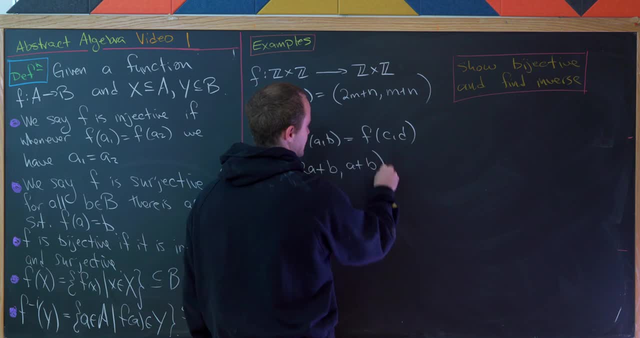 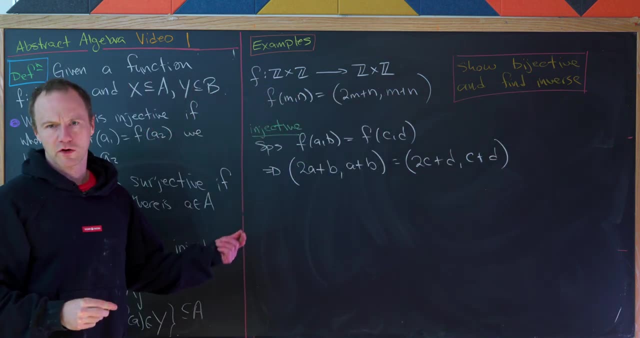 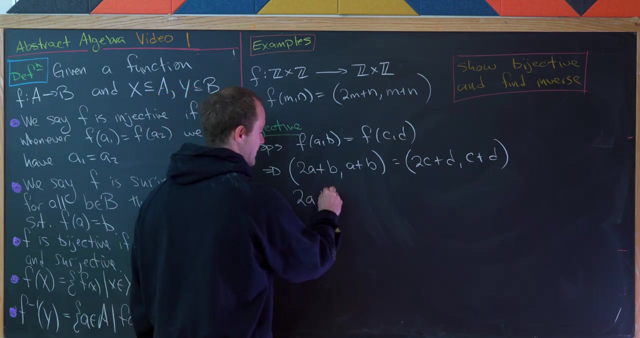 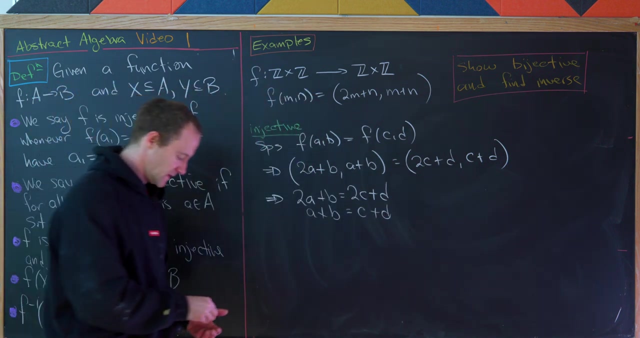 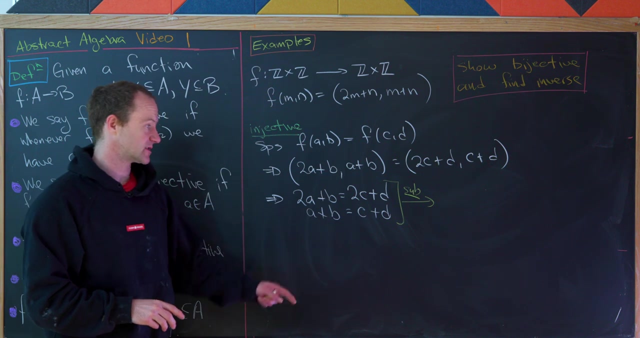 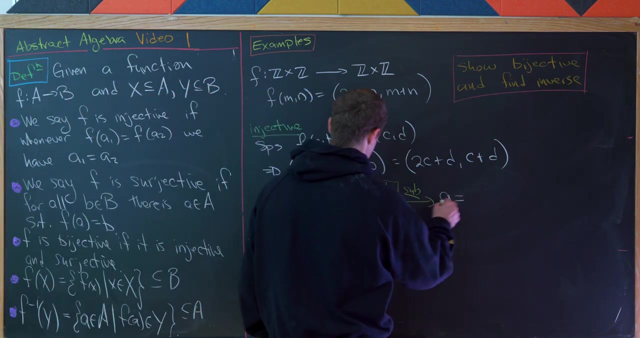 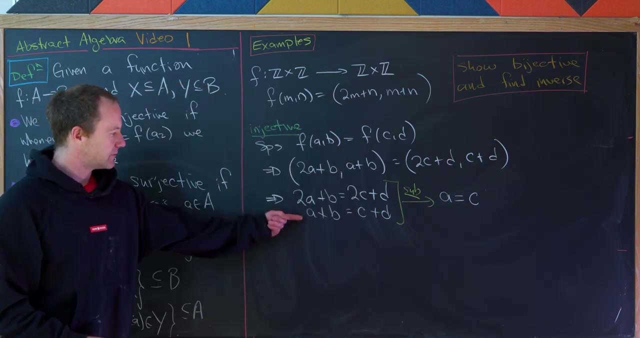 ... b comma a plus b is the same thing as the ordered pair 2c plus d c plus d. But now ordered pairs are equal if and only if both entries are equal. So that gives us a nice system of equations. 2a plus b equals 2c plus d from equating the first entry. And then we also have a plus b equals c plus d from equating the second entry. But now check it out. We can subtract. So if we subtract these two equations the b's cancel on the first equation and the d's cancel on the second equation. And we're left with 2a minus a which is a and 2c minus c which is c. So we immediately see that a is equal to c. But then plugging that into the second equation. 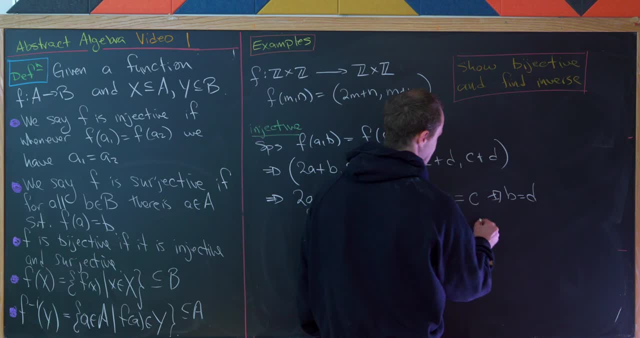 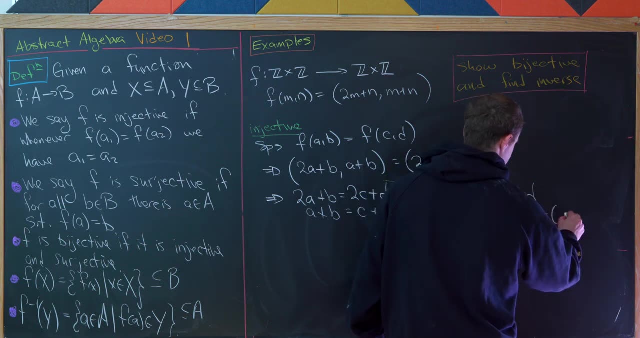 We also see that that leads to b equals d. But then if a is equal to c and b is equal to d then that means that a comma b equals c comma d. But that's exactly where we needed 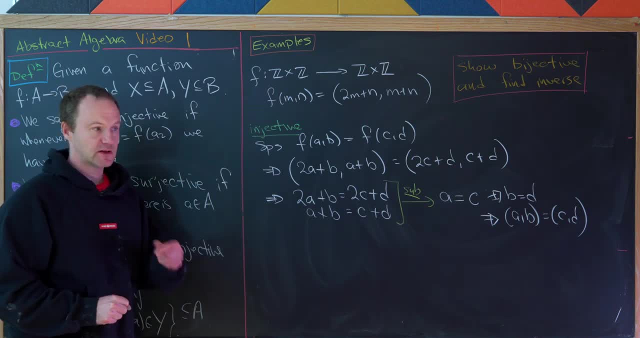 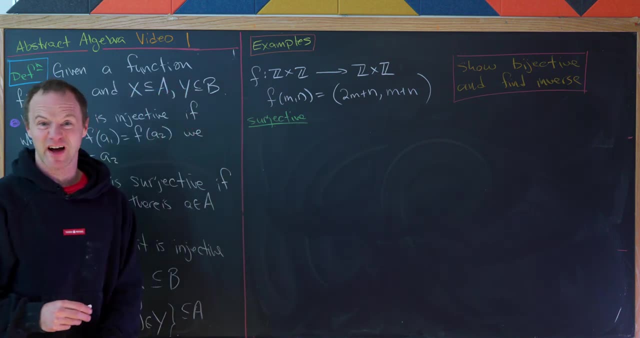 to end up for this thing to be injective. So now let's show it's surjective. Okay so to show it's surjective let's take an arbitrary element of the codomain and then find something that maps onto it. 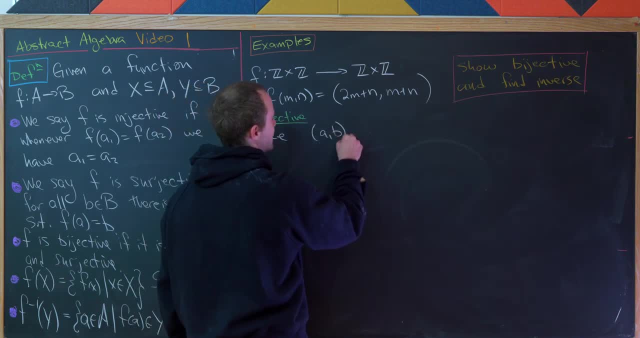 So let's like I said take 1 we'll call it a comma b from z cross z. And then we'll want to solve the equation f of 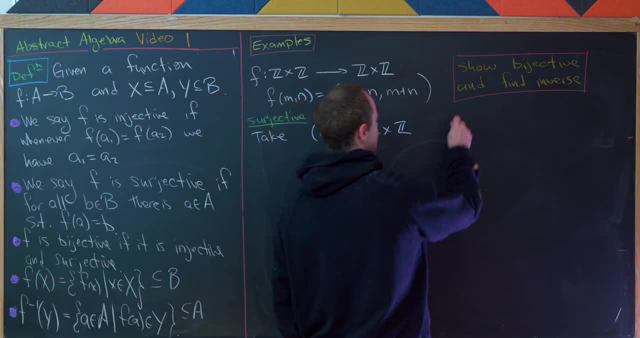 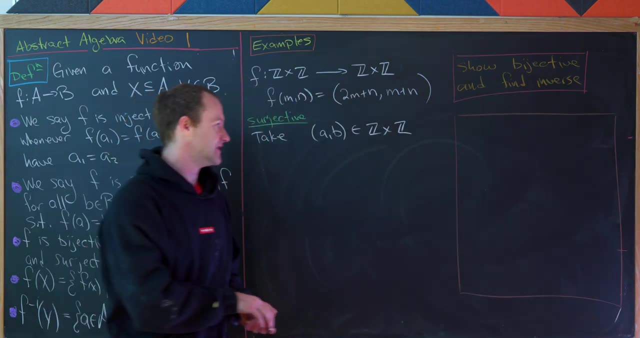 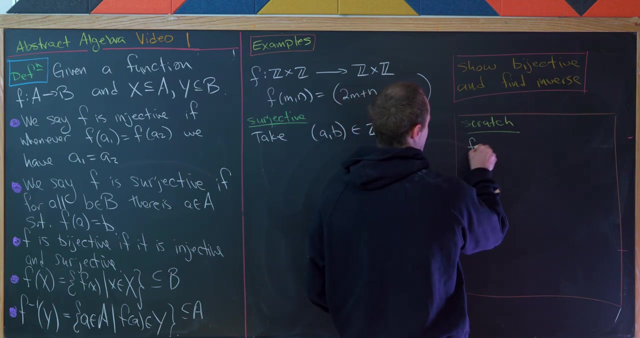 m n equals a comma b. And generally you do this in a scratch work and then final version you know kind of order here. So let's say this is our scratch work over here where we do the side calculation. Okay so let's look at f of m n equals a b. And let's see what happens. So if f of n is equal to b that means that m and n have to be in terms of a and b of course. 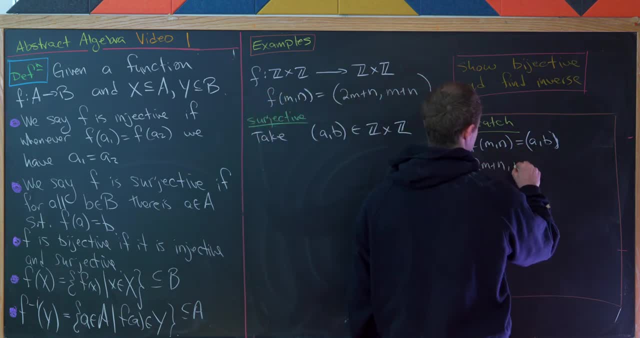 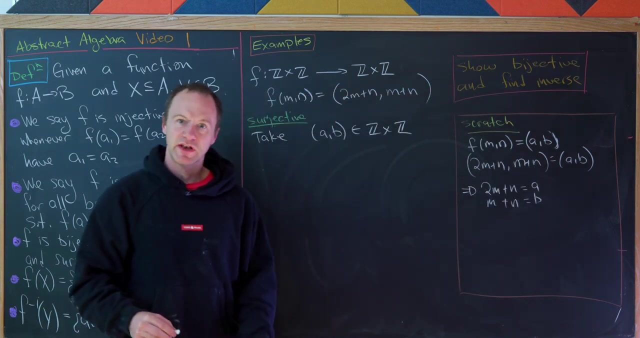 Okay. So let's see. That means we have 2 m plus n comma m plus n equals a comma b. But that means that we have a system of equations 2 m plus n equals a. And then m plus n equals b. 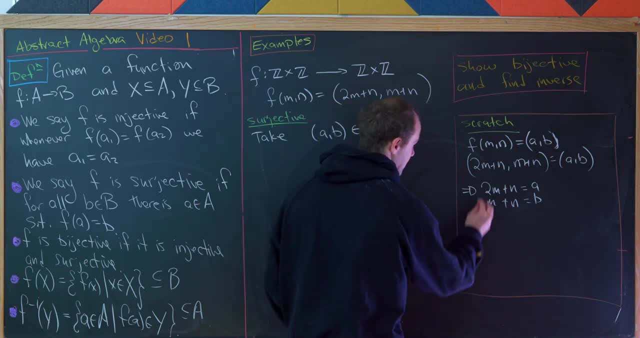 But now we can subtract these just like before and we'll get some nice simplification. So if we subtract these. 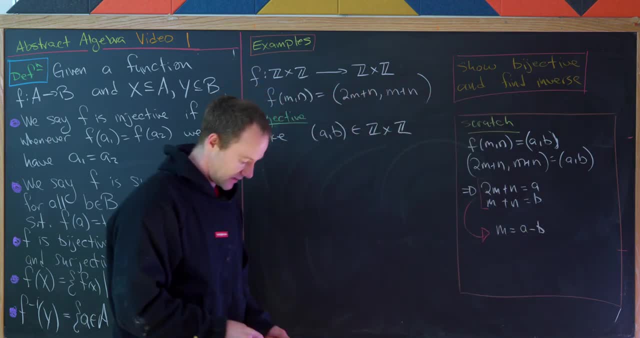 see that m is equal to a minus b okay but then rolling that into the second equation we get 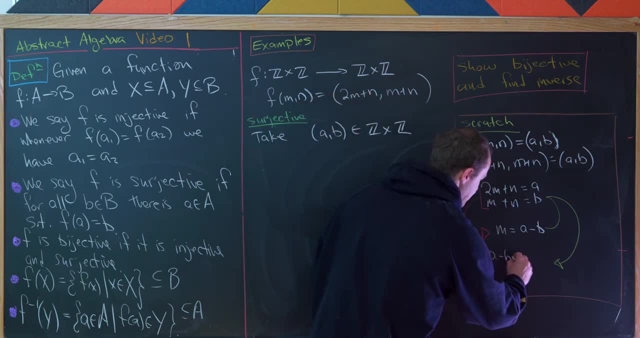 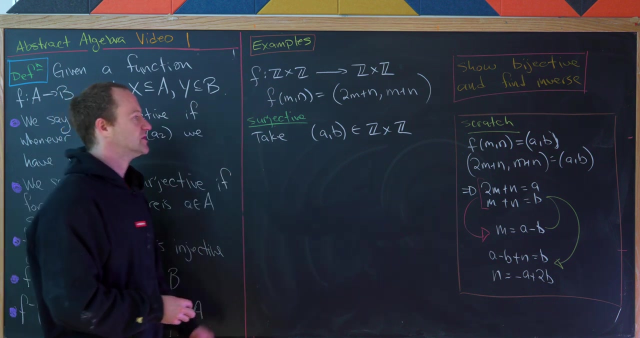 something nice we'll have a minus b plus n equals b which means we have n equals let's see what will it be minus a plus 2b so there we have m and n in terms of a and b okay so how do we finish this 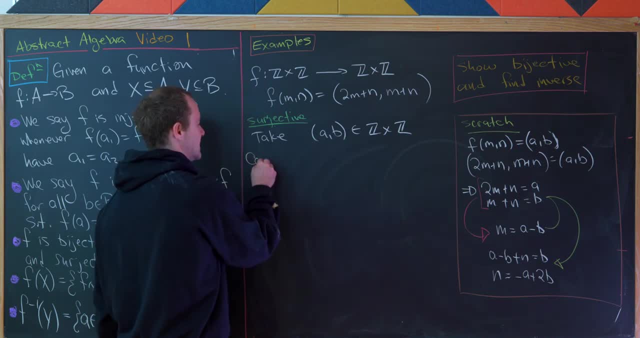 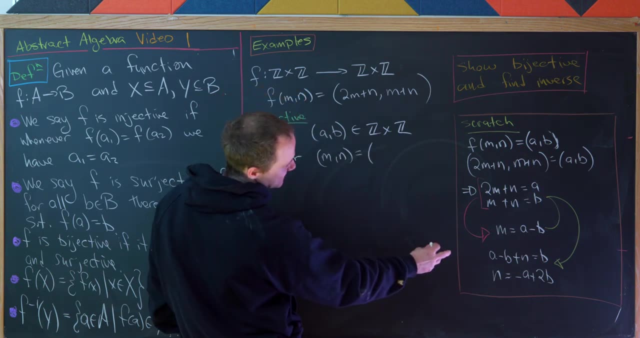 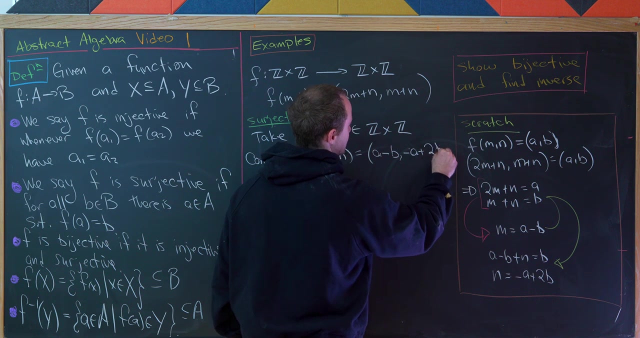 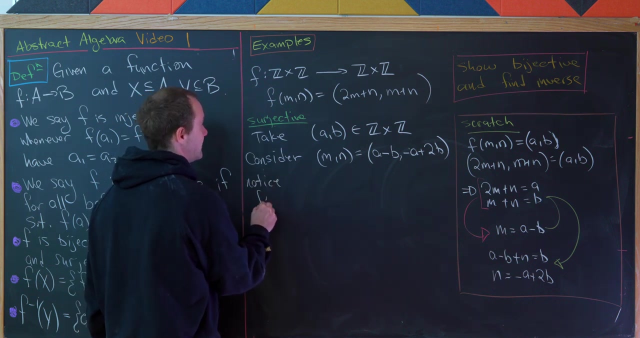 thing off so we take like i said a b from z cross z and then let's consider our m comma n equal to let's see what we found over here so a minus b and then minus a plus 2b great and then we would say something like this let's notice that f evaluated at this m n is the same thing as this f evaluated at this m n is the same thing as this f evaluated at this m n is the same thing as this 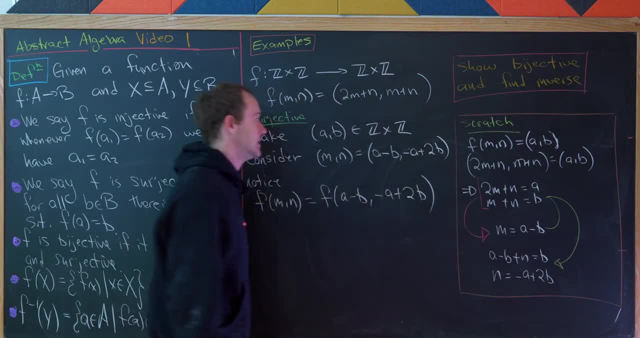 f evaluated at a minus b minus a plus 2b but that's going to be equal to 2 times a minus b 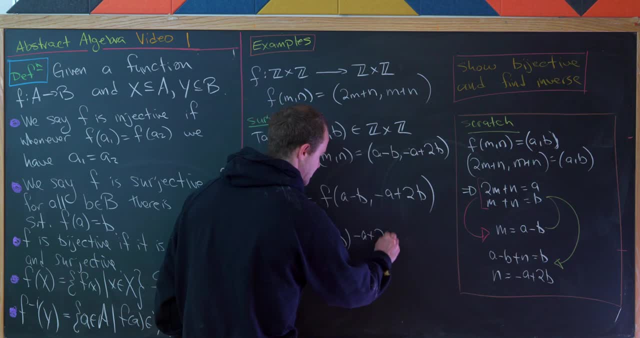 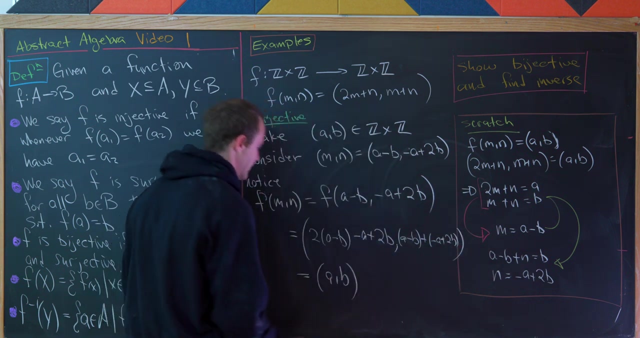 and then minus a plus 2b you know based off this formula right here and then the sum of these two so that's going to be a minus b plus minus a plus 2b but what we'll see is that simplifies down to a comma b so we found a pre-image for the sum of these two so that's going to be a minus b element a comma b which means we have finished our surjectivity proof so now we know it's 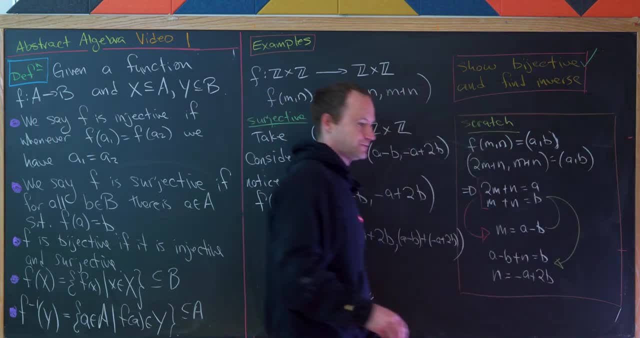 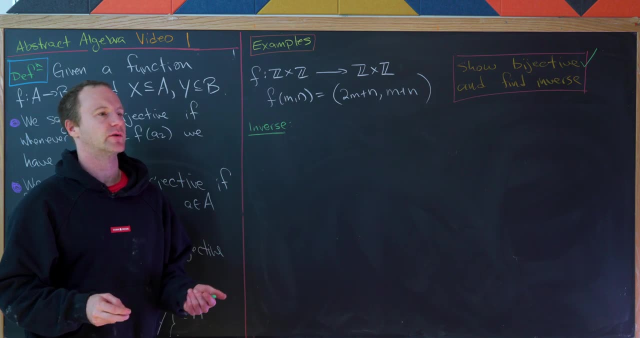 bijective so let's maybe put a check mark over here now let's work to find its inverse so we're going to use a trick to find its inverse from linear algebra that's generally a prerequisite for this type of course so i don't feel too bad using that that being said we could essentially guess the inverse from our surjectivity calculation but i think it's good to add this in here 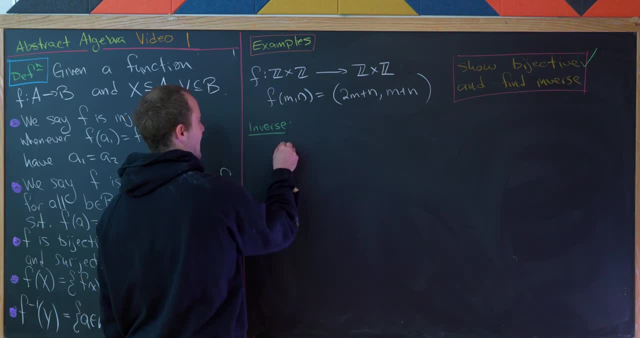 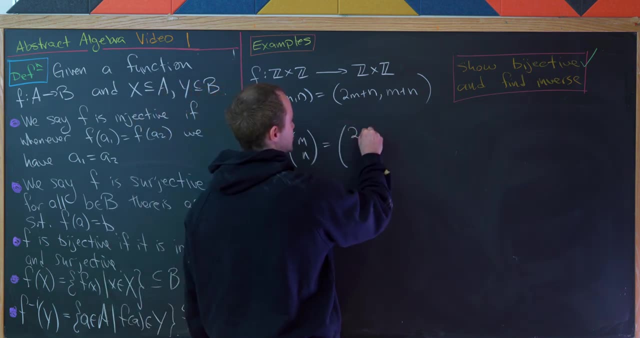 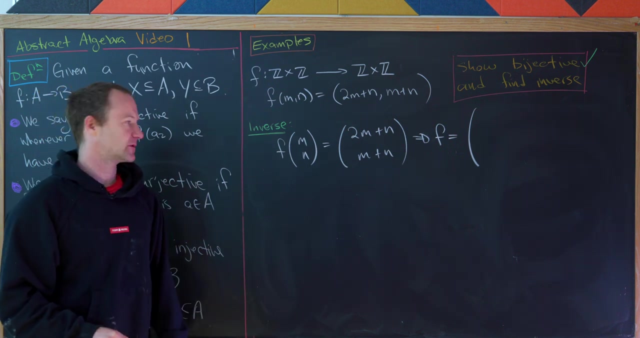 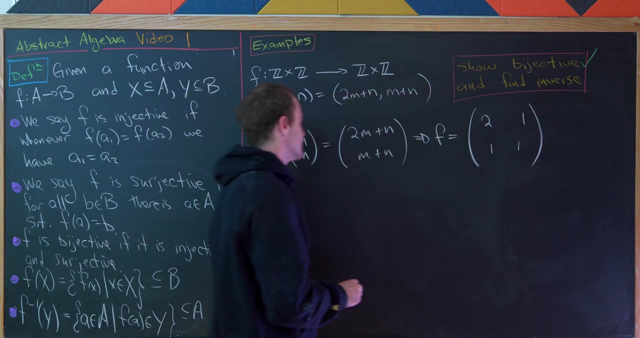 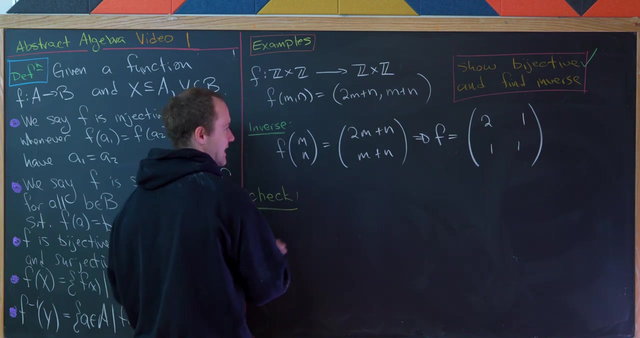 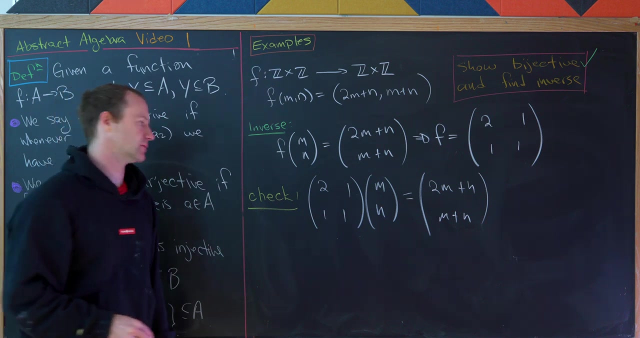 okay so let's rewrite this equation as a vector equation so let's say f takes the vector m in and gives us the vector 2m plus n m plus n but what does that mean that means our function f is essentially equal to a matrix notice this is a linear transformation every linear transformation can be represented as a matrix and that matrix in this case is 2y2n 1 1 and then how do we know this well let's check that this makes sense so let's multiply this matrix 2 1 1 1 onto m n and note that we get exactly what we want up here 2m plus n and then m plus n and that's of course using our standard matrix vector multiplication we swivel this first 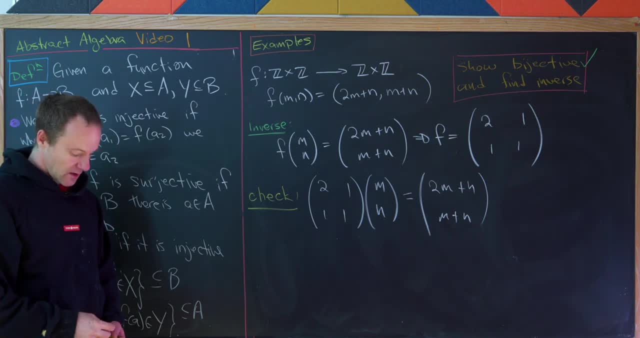 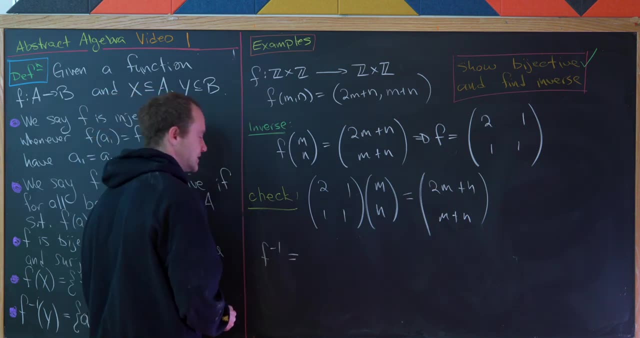 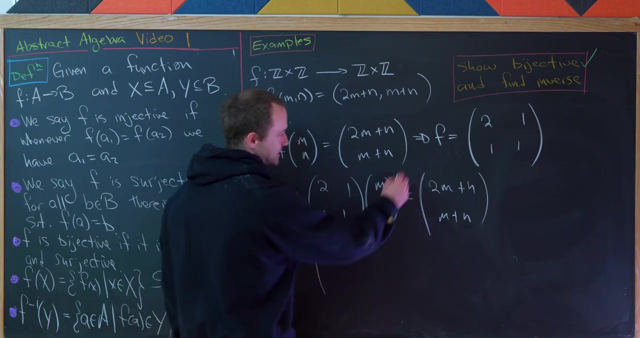 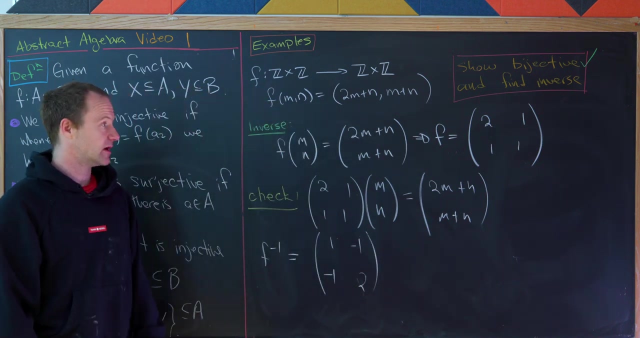 row into the column and add and so on and so forth but we also know how to find the inverse of 2x2 matrices fairly easily so we can use the rule for that so f inverse will be equal to let's recall we have 1 over the determinant in this case the determinant is 1 so that's easy and then what do we do after that well we swap the diagonal entries and then we negate the off diagonal entries so that's the standard rule for taking the determinant of a 2x2 matrix okay but now we 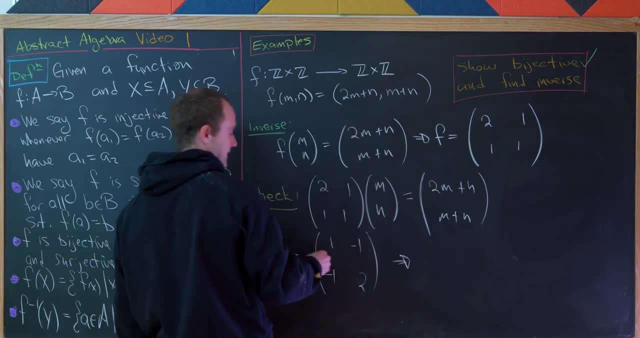 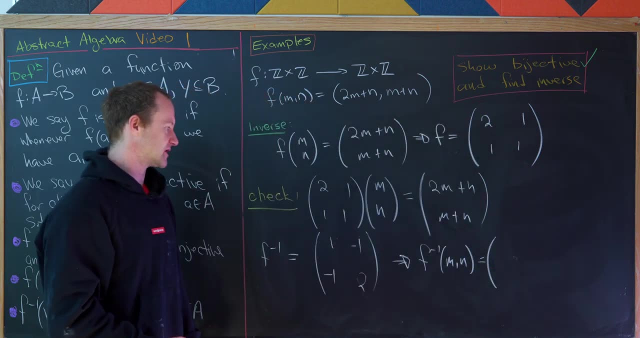 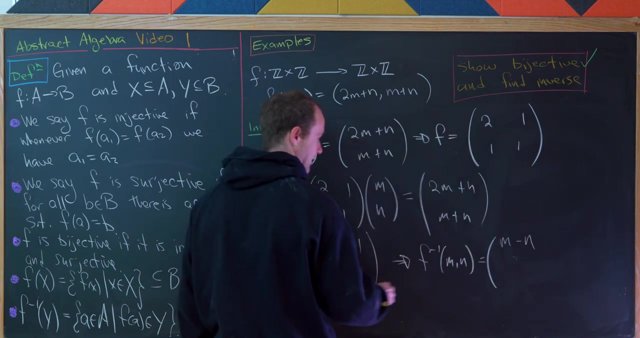 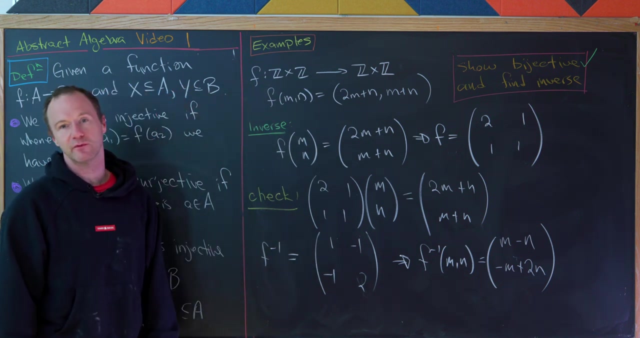 can put this back into our form like this and we'll see that f inverse evaluated at m n is equal to well we just multiply this onto the vector m n and we'll see that we get what m minus n and then it'll be minus m plus 2n and that's suspiciously familiar to something that we had before so like i said there's a lot more to do with functions but that's all where 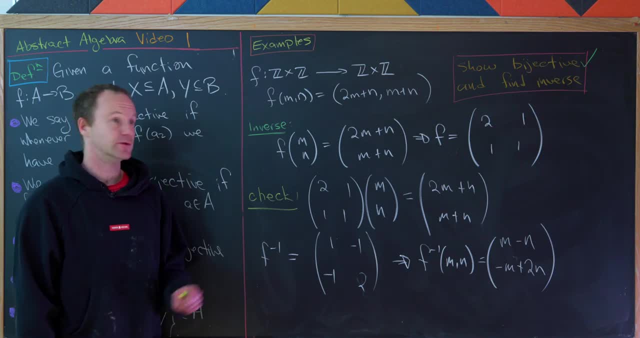 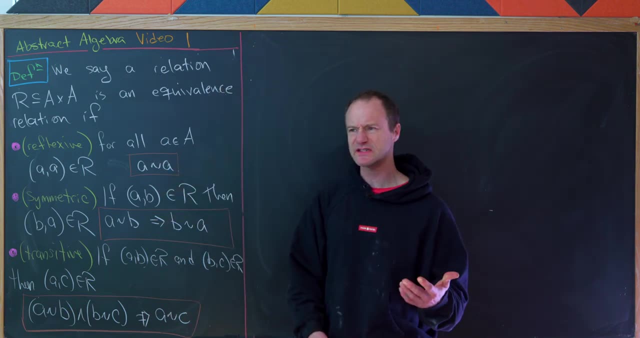 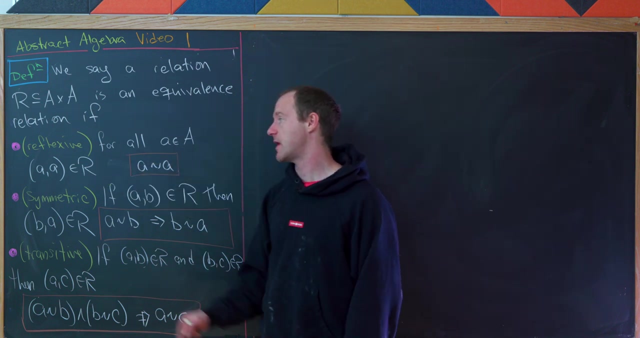 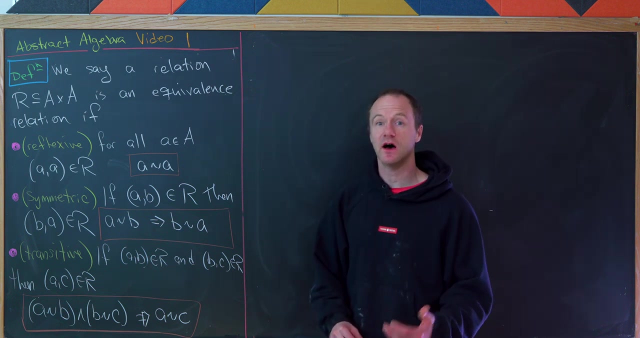 we are going to do i urge you to review more if you need to now we're going to look at the notion of an equivalence relation so let's recall that we say a relation on a cross a so that's between a set and itself is an equivalence relation if it satisfies three important properties so the first one is called reflexivity and that says for all a in a a comma a is an r so in other words a is related to itself and then it also has to be symmetric so that means if a comma b is an r then b comma a is an r or 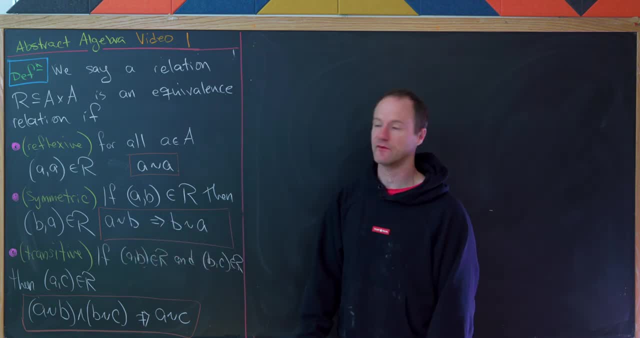 a tilde b implies b tilde a that would be another way of writing that down it also has to satisfy transitivity and that says if a comma b is an r and b comma c is an r then a comma c is an r 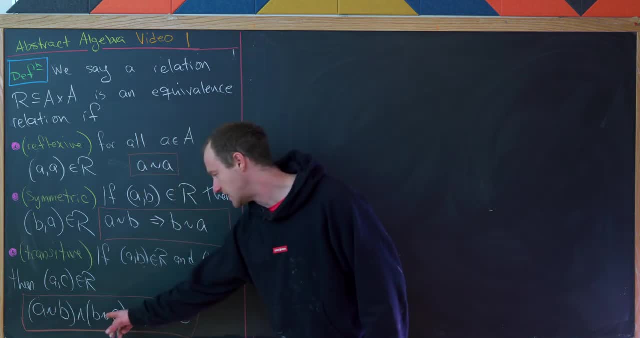 so in other words if a is related to b and b is related to c that implies a is related to c 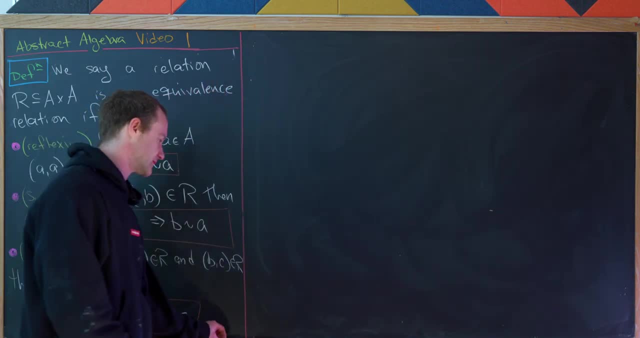 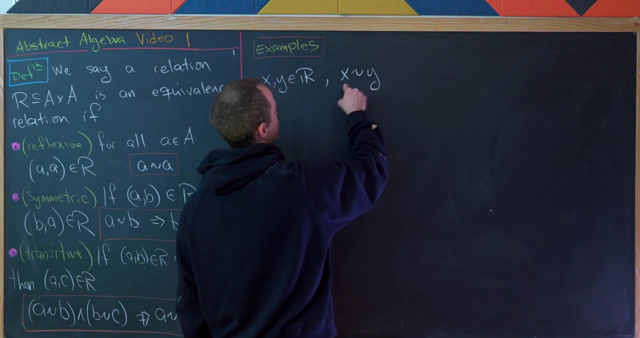 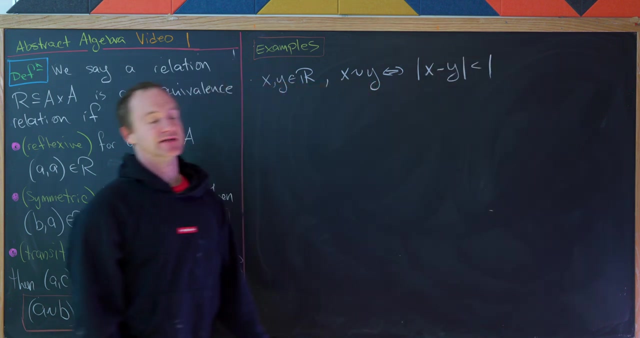 okay so let's look at a couple of examples so let's say that x and y in the real numbers are related so in other words x tilde y if and only with if the absolute value of x minus y is equal 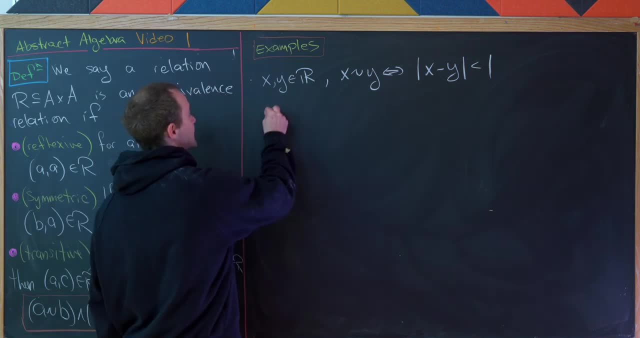 to one so we will show that this is both reflexive and symmetric so notice that it is reflexive because we have the following x tilde x 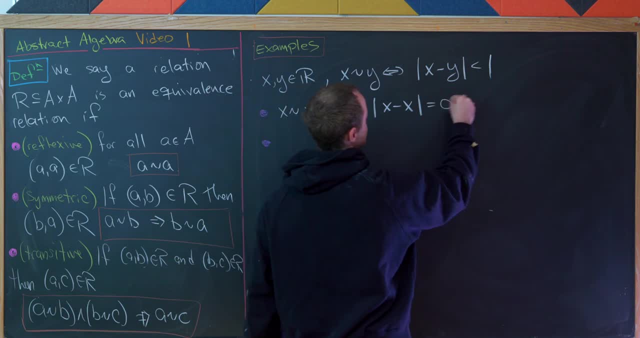 because the absolute value of x minus x equals zero which is most definitely less than one 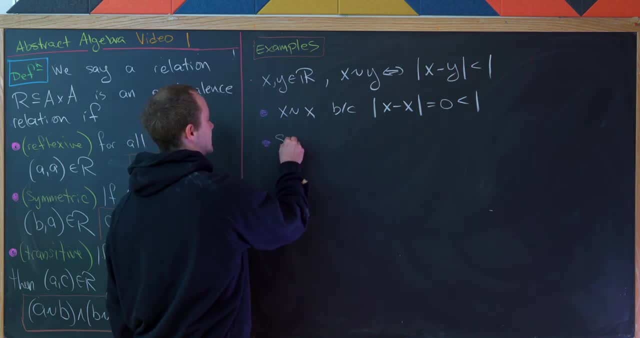 now let's show that it's symmetric so let's suppose that x is related to y but that means 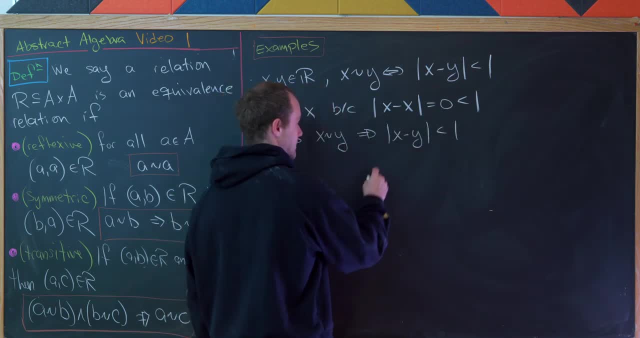 that absolute value of x minus y is less than one but that means that the absolute value of y minus x is less than one so let's show that it's symmetric so let's suppose that x is related to y 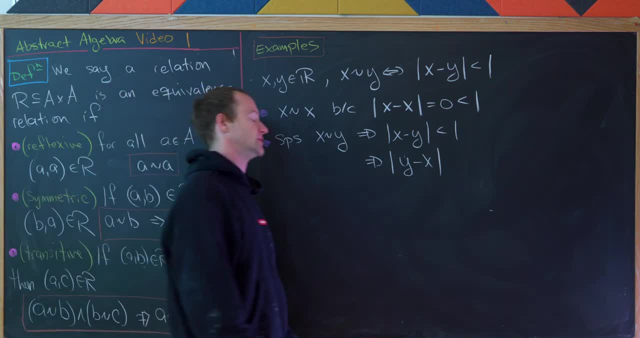 less than one essentially because the absolute value of negative one is equal to positive one 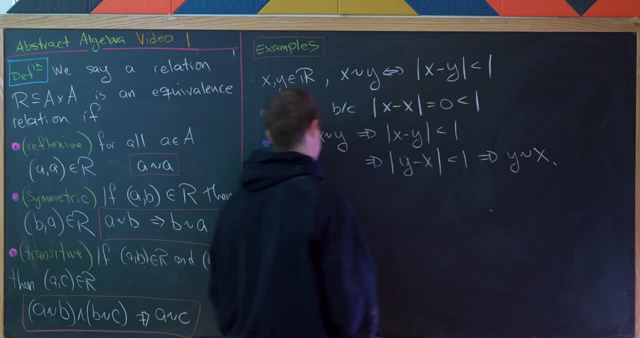 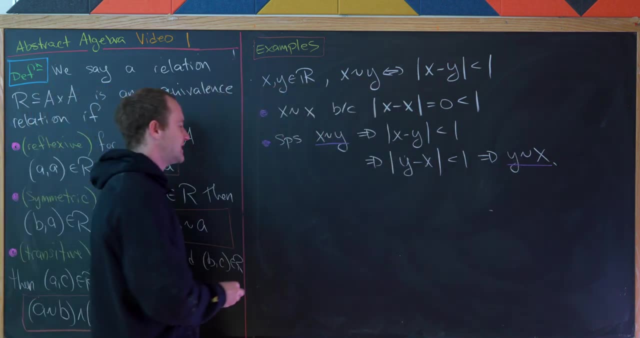 but that means that y is related to x so let's see starting here and ending here is what we needed to prove symmetry but this thing is not transitive and we can check it's not transitive 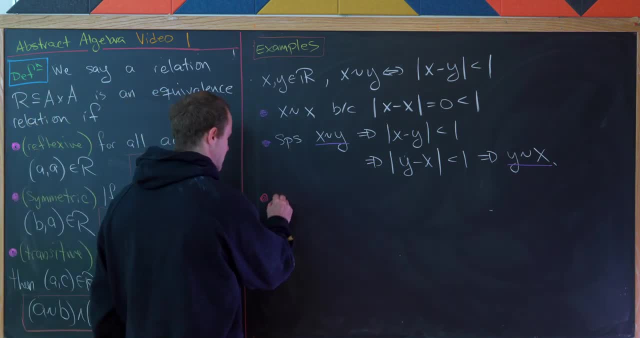 by an example and that's like this note that we have zero is related to three quarters 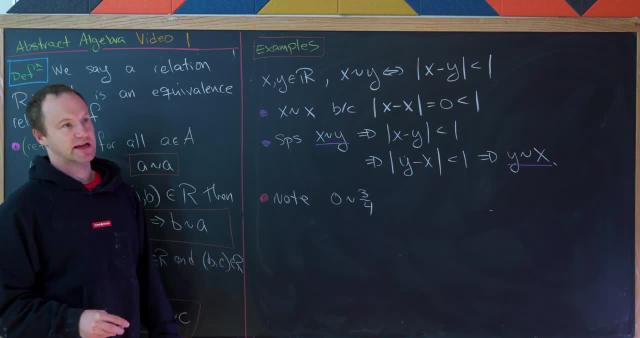 that's because three quarters minus zero is equal to three quarters which is less than one 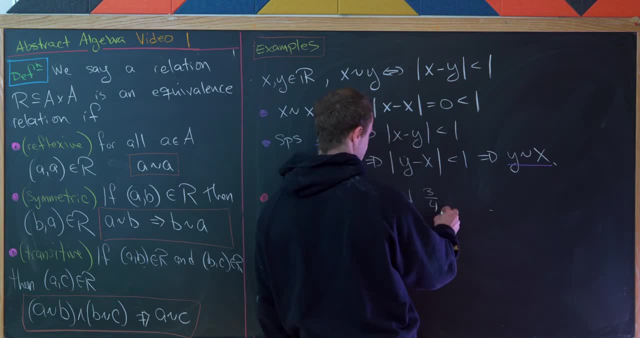 and we also have three quarters is related to one and a half and in other words three halves 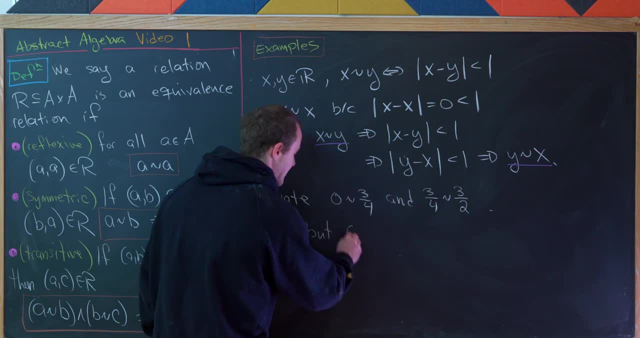 that's because of the same reason but we have zero is not related to three halves that's because 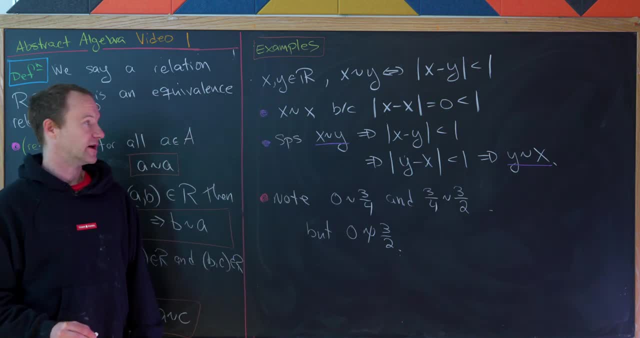 zero and three halves are not within one of each other so how could we maybe fix this 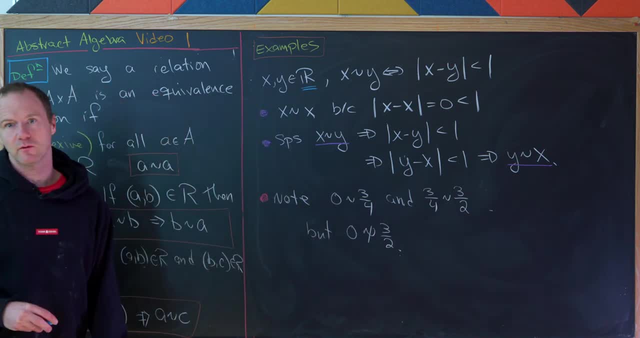 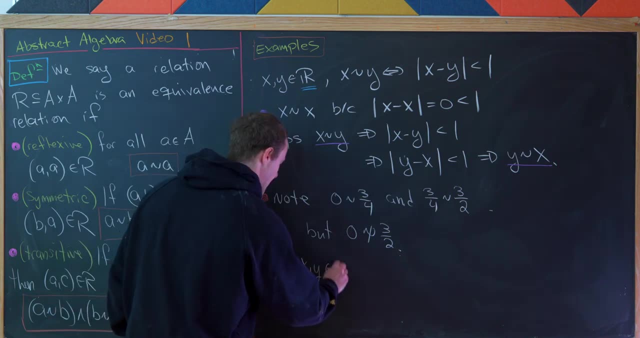 well we could fix this by changing the set that we're working over so let's maybe do that down here so let's notice that if if we take x comma y in the integers then we do get transitivity and 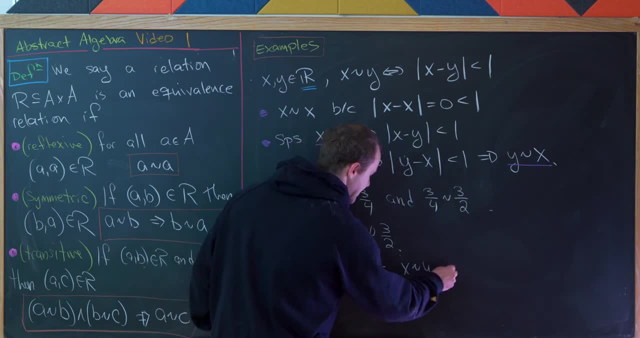 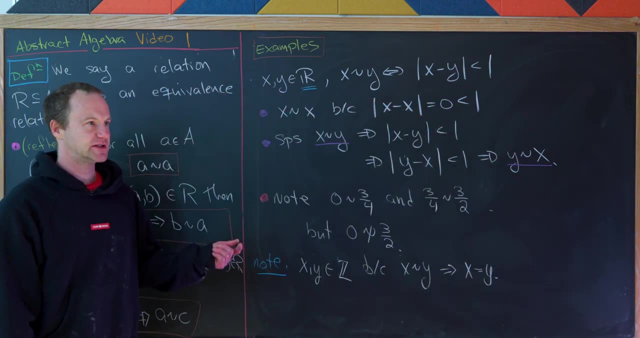 that's because if x is related to y then x is equal to y and that's simply because there are no integers that are less than one away from each other because it's not Technologies ofportation. less than one away from each other unless they're the same thing. 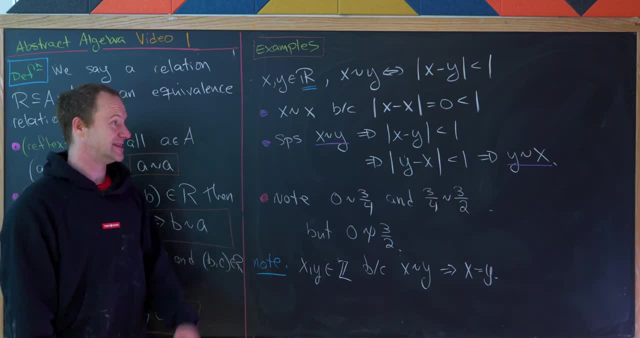 So I'll let you think over that if you need to, but I think this provides a nice example of a non-equivalence relation 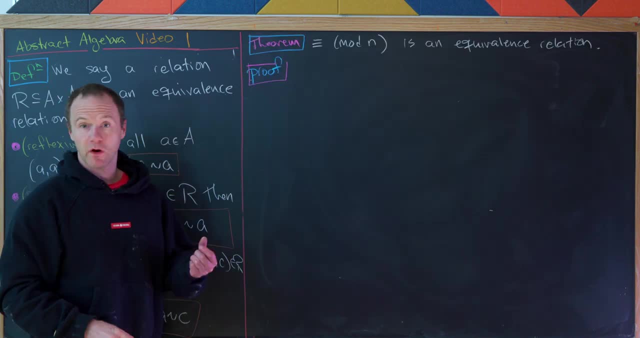 that becomes a very simple equivalence relation quickly. So our last result will be to prove that congruence mod n is an equivalence relation. 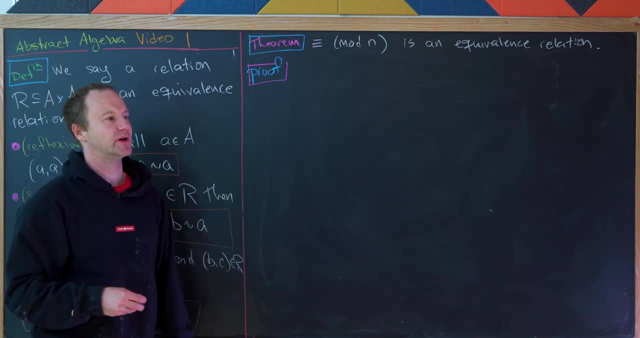 So you saw this proof before in an intro to proofs class, but we're gonna review it here as we'll work with congruence mod n quite a bit in this course. 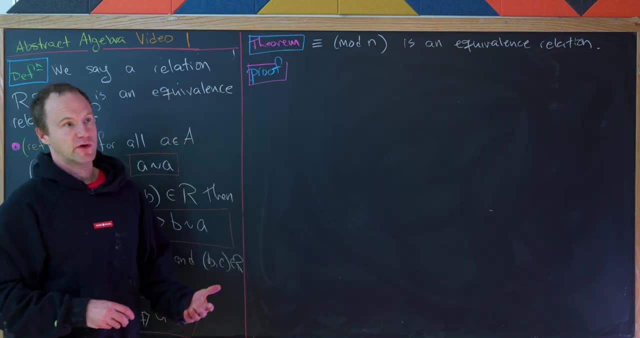 Okay, so let's first prove that we have reflexivity. 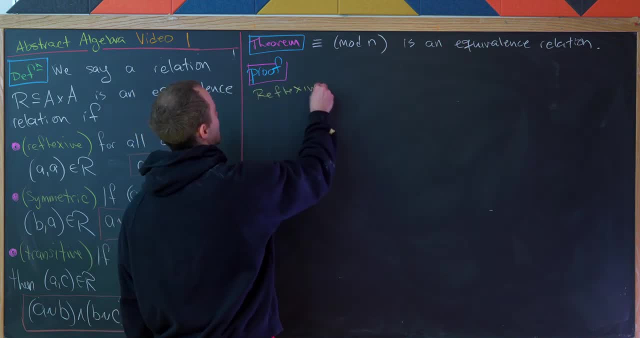 Okay, so let's maybe see how that might go. 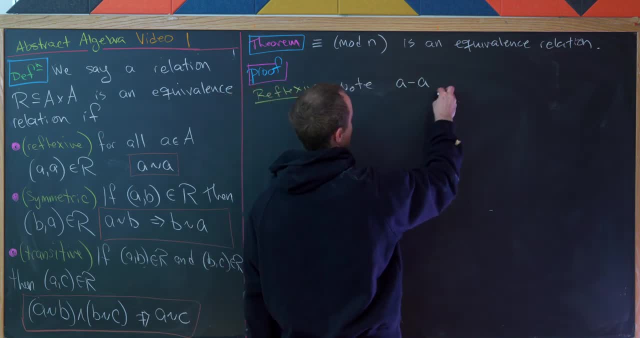 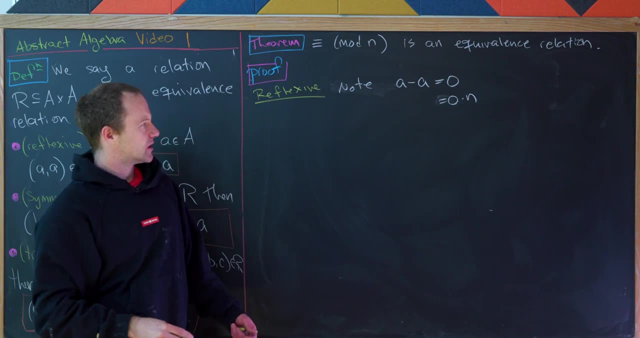 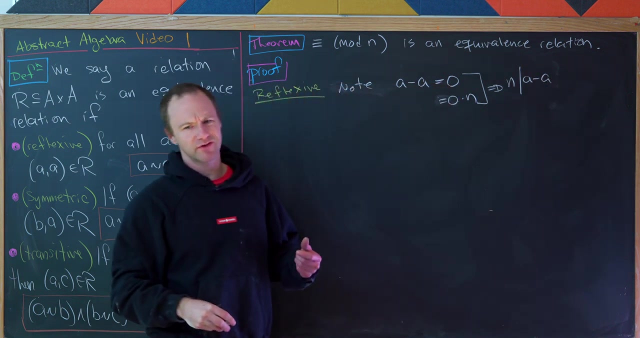 So let's note that a minus a is equal to zero, but zero is equal to zero times n. So what does that mean? So that means that n divides a minus a. So here we're using some definitions that come from this. This is from that previous class. 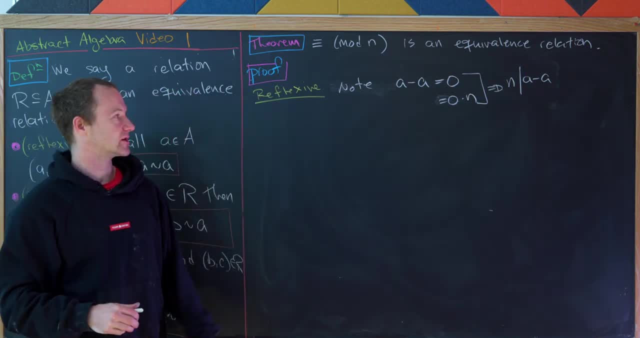 But we can't review everything, so that's just the situation here. 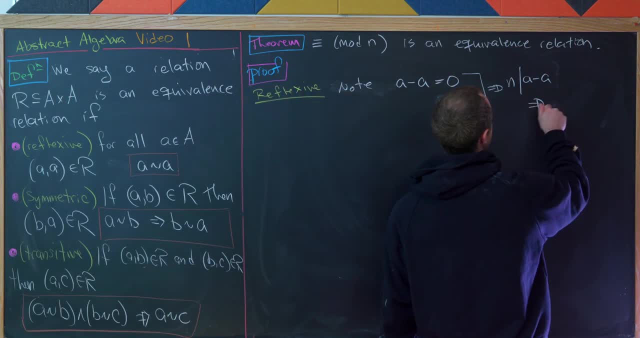 But if n divides a minus a, that's exactly the definition of saying that a is congruent to a modulo n. And now we're good to go. 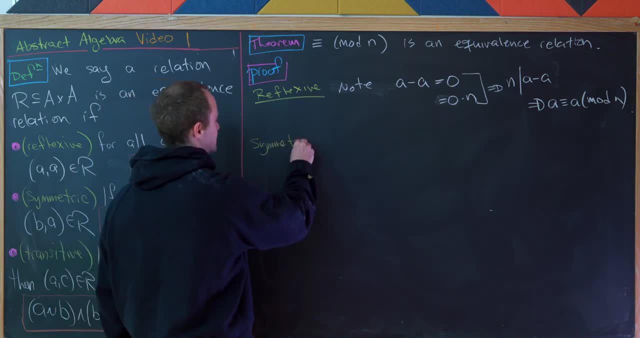 Okay, so now let's prove symmetry. Okay, so how might that go? 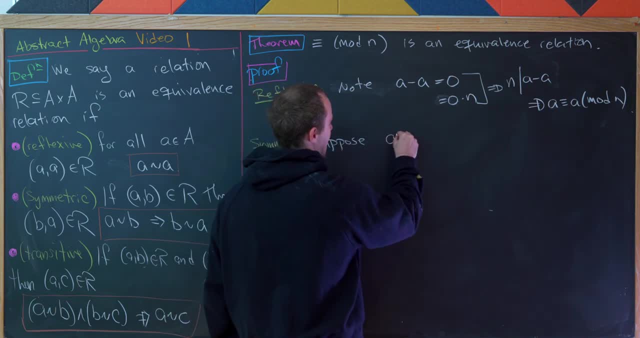 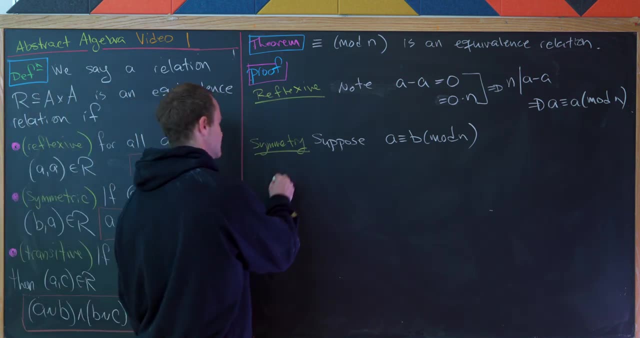 Well, we need to suppose that a is congruent to b mod n, and hopefully get to the point where b is congruent to a mod n. 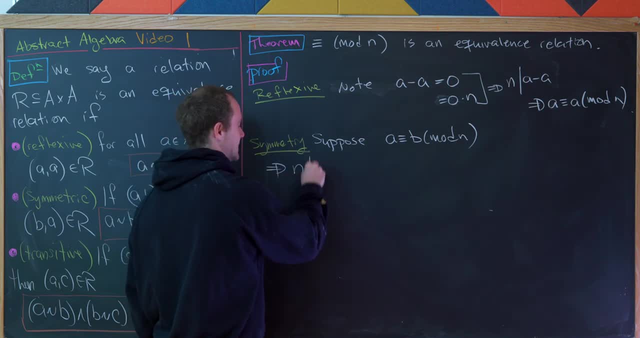 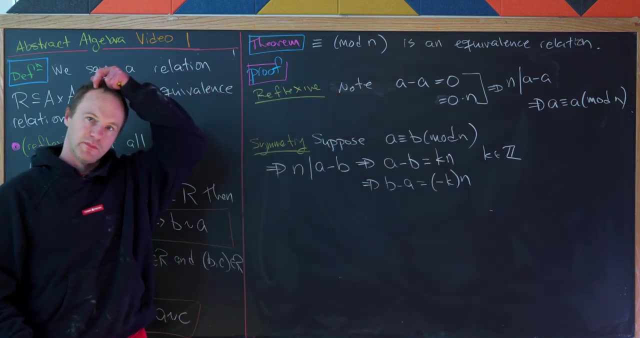 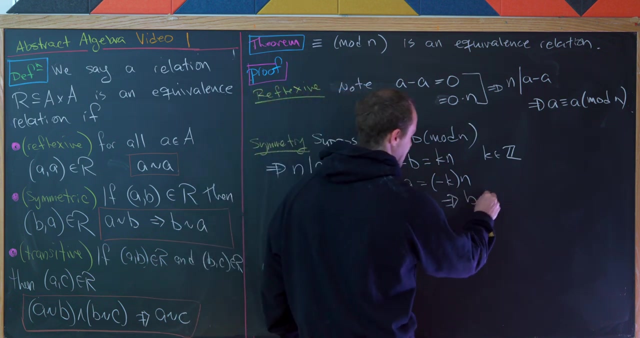 So unwrapping the definition, this means that n divides a minus b. But that means that a minus b is a multiple of n. Maybe we'll say that it's equal to k times n for some integer k. But we can just multiply both sides by minus one, and we have b minus a is equal to minus k times n. But that means that n divides b minus a. But in turn, that means that b is congruent to a modulo n. 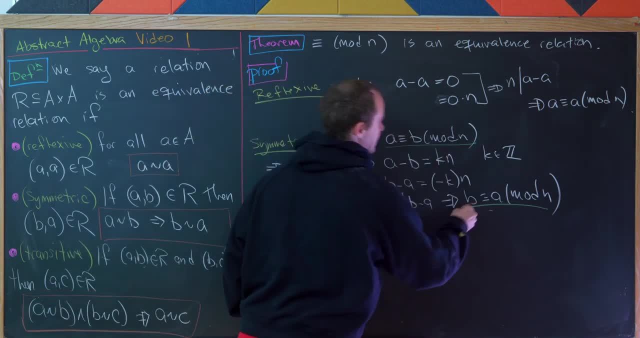 So the fact that we were able to start right here and end right here means that we have symmetry of this relation. 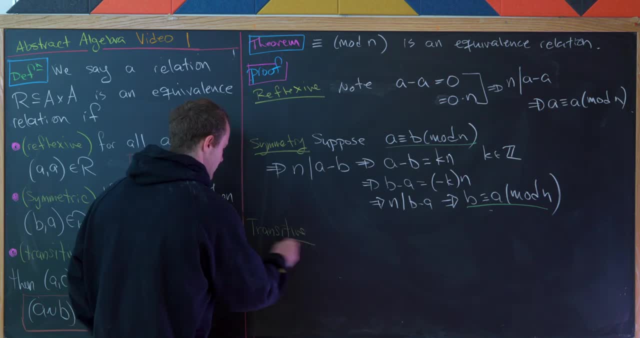 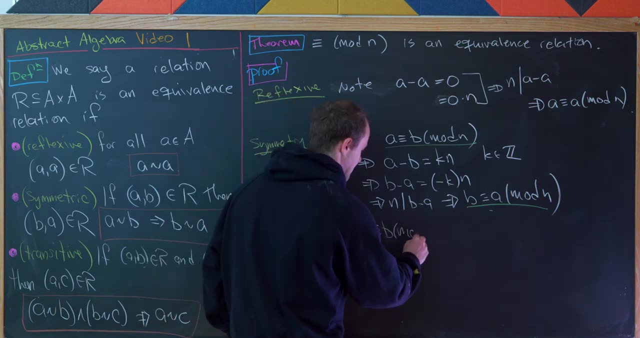 Now let's finish this by proving transitivity, which means we need to suppose two things. So let's suppose that a is congruent to a mod n. So let's suppose that a is congruent to a mod n. So let's suppose that a is congruent to a mod n. And that b is congruent to c modulo n. 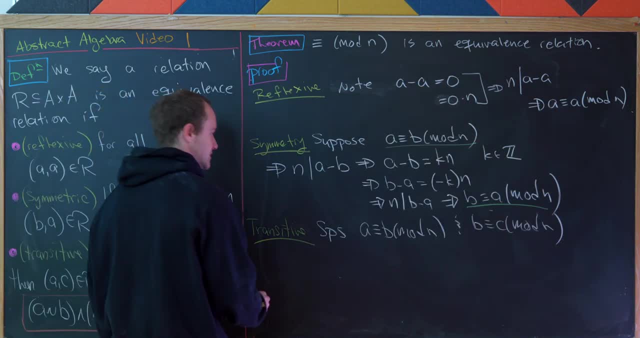 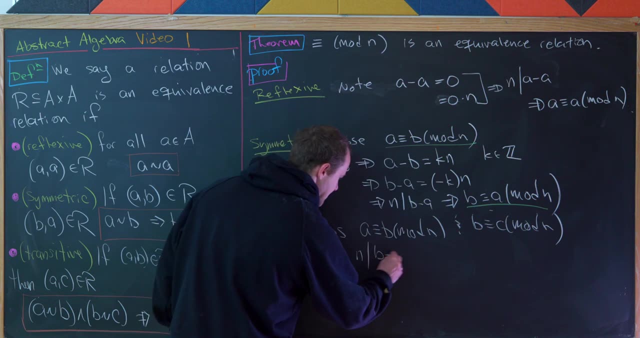 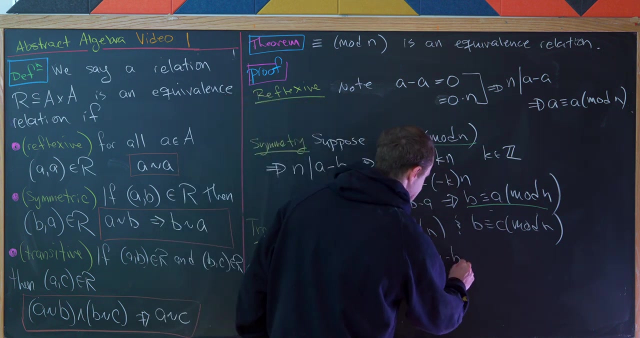 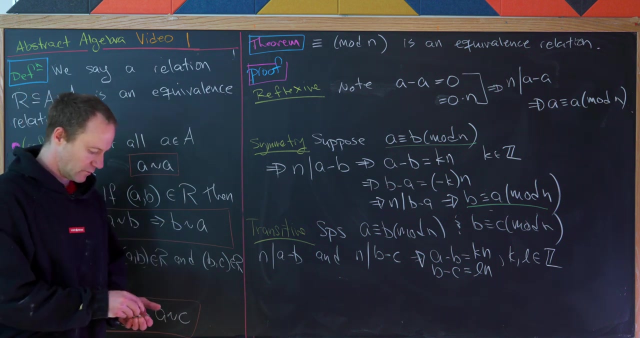 Okay, so now let's unwrap both of those definitions. So that means that n divides a minus b, and n divides, let's see, b minus c. But unwrapping further, that means that a minus b is equal to k times n, and b minus c is equal to, something we'll call l times n. And this is for integers k and l. But what should we do from here? Well, let's take these two equations and then add them. 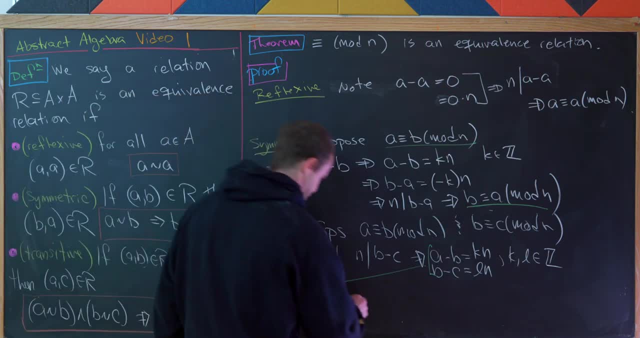 So let's see, if we add those two equations, the b's cancel, and we're left with a minus c is congruent to k plus l, or is equal to k plus l times n. 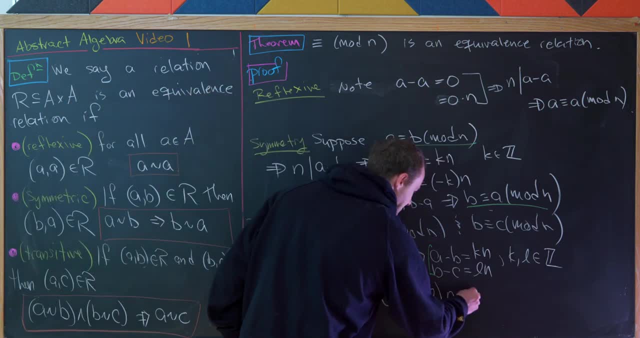 l times n. But that means that n divides a minus c. 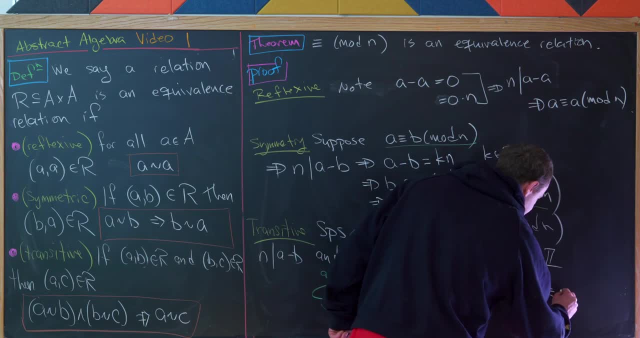 But finally, that means that a is congruent to c modulo n. 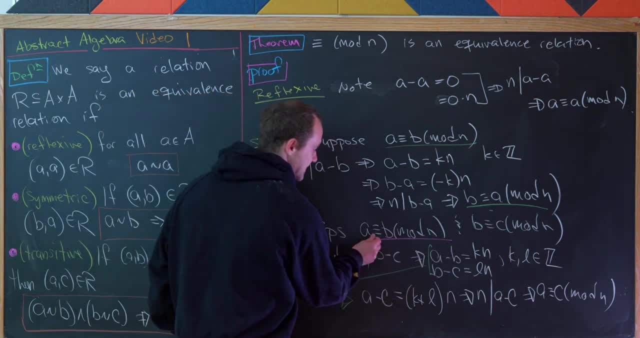 So now the fact that we were able to start with these two assumptions and end with this assumption means that we do have transitivity. 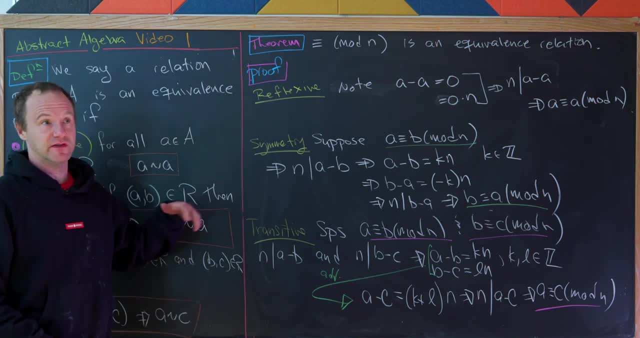 Okay, so what are some things that we didn't quite cover in this lecture that you might wanna remind yourself of to succeed in this course? 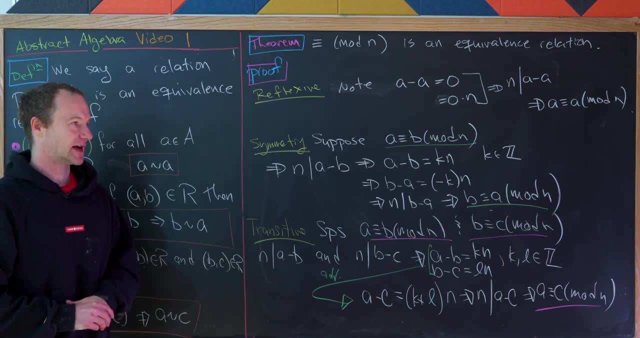 Well, I would say you wanna look up the notion of an equivalence class. So we did quite a bit with that in the intro to proofs class that, again, like I have a bunch of videos for. So I would check those out if you need that sort of review. But the notion of an equivalence class goes hand in hand with an equivalence relation. 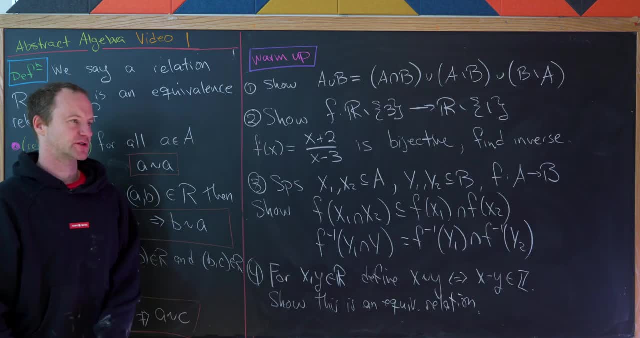 Okay, so now I'm gonna leave you with some warmups. So I've got four warmup exercises for you. 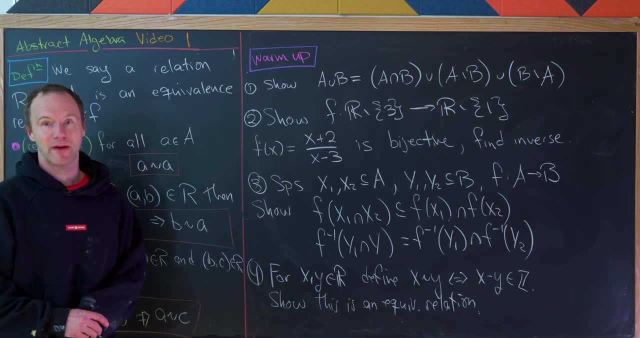 Based off what we talked about today and just like general background information that it might be nice to review. 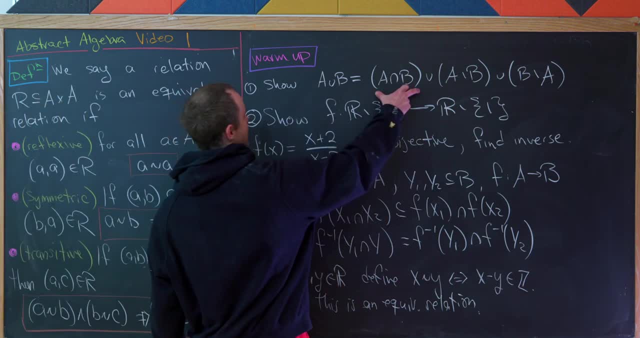 So the first is that A union B is the same thing as A intersect B union A minus B union B minus A. 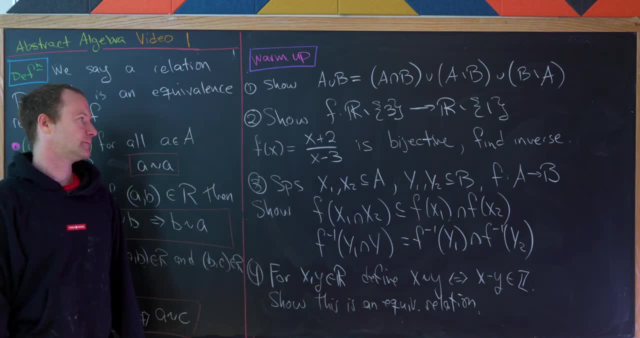 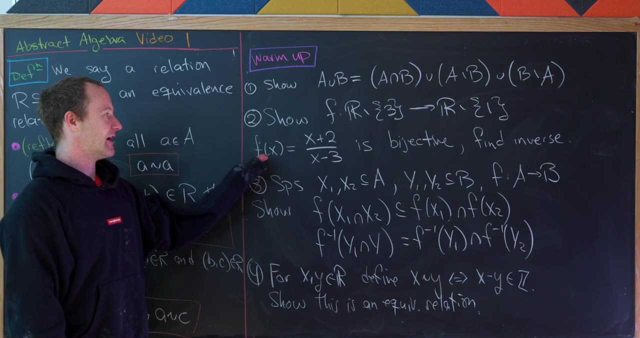 So you might need to look up the set subtraction for that. Next, let's define a function from the real numbers minus three to the real numbers minus one by F of X equals X plus two over X minus three. Show that function and find its inverse. 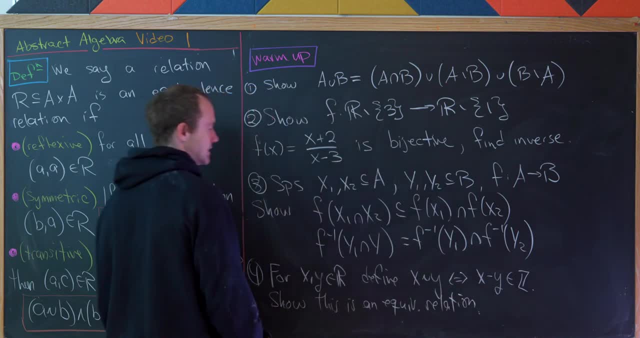 Next, let's say that we've got a function from A to B and we have two subsets of the domain and two subsets of the co-domain. 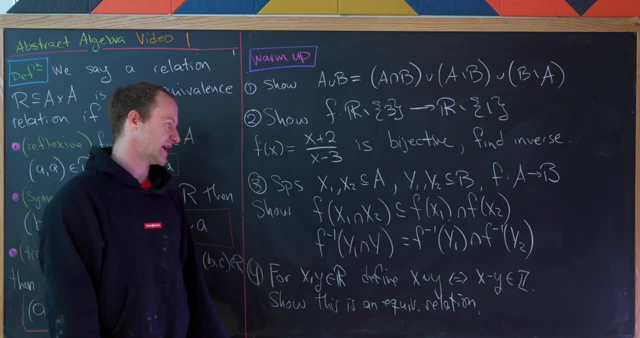 So let's show that the image of X one intersect X two is a subset of the intersection of those two images. 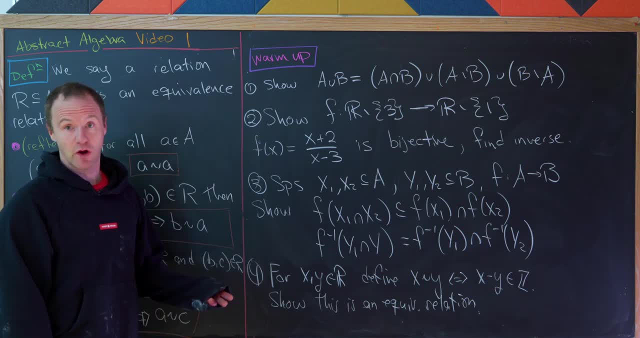 And then maybe a followup question is, does equality hold in this case? Or is it possible that this is a proper subset? 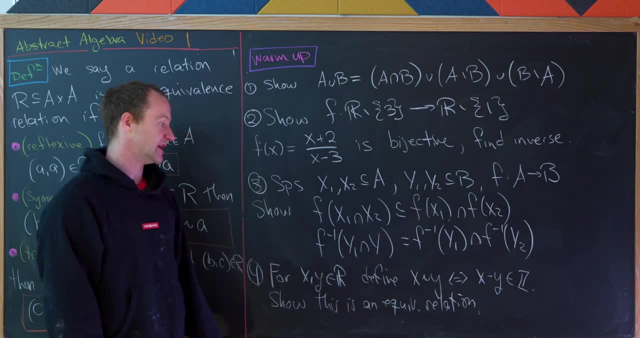 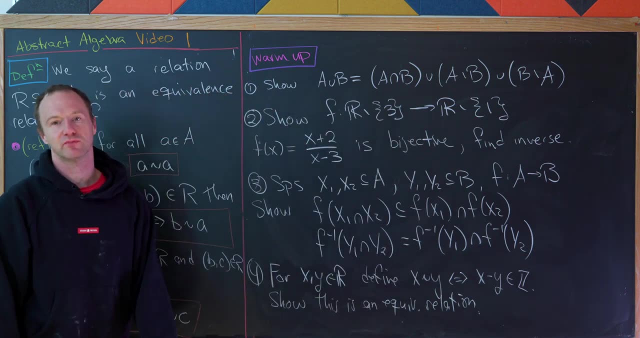 Next, show that the real numbers minus two over X two is a proper subset. Next, show that the preimage of the intersection of Y one and Y two is the same thing as the intersection of the two corresponding preimages. 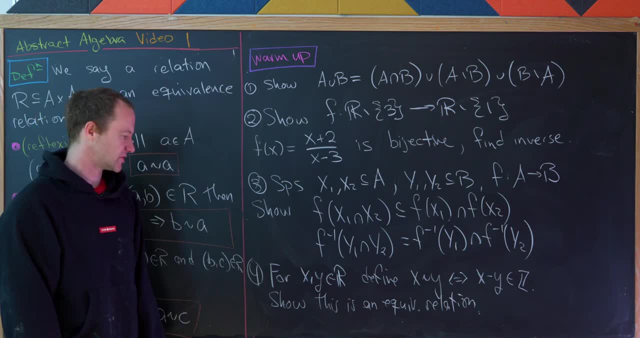 So in fact, preimage is kind of nicer with set operations. 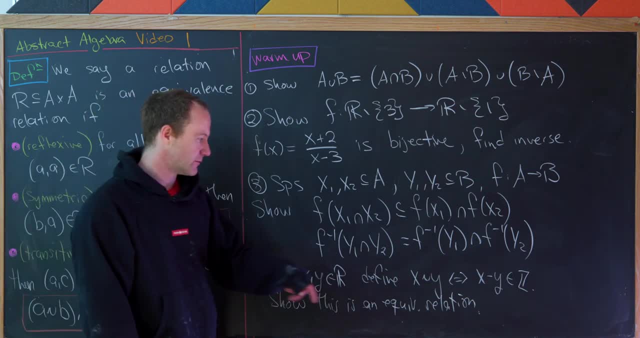 Then finally, let's define a relation on the real numbers by X is related Y if and only if X minus Y is an integer. 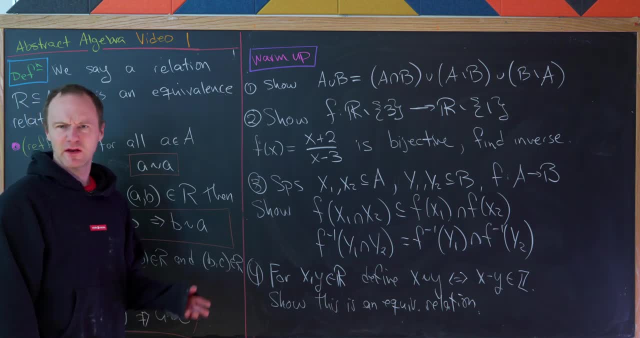 Then let's show that that is an equivalence relation. And then maybe also describe 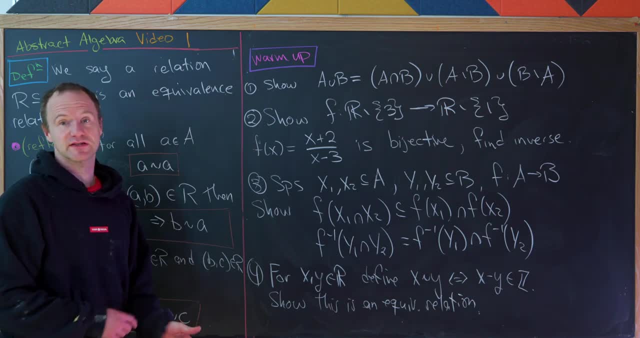 describe the equivalence classes and that's a good place to stop. 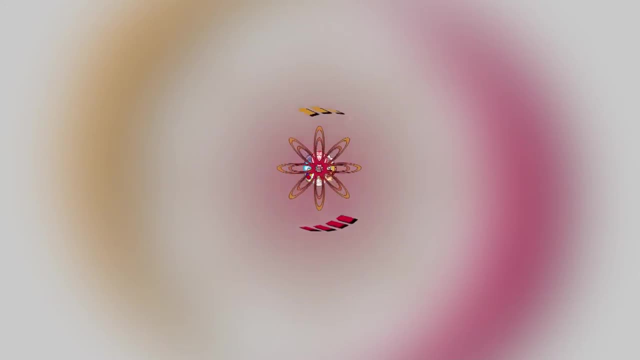 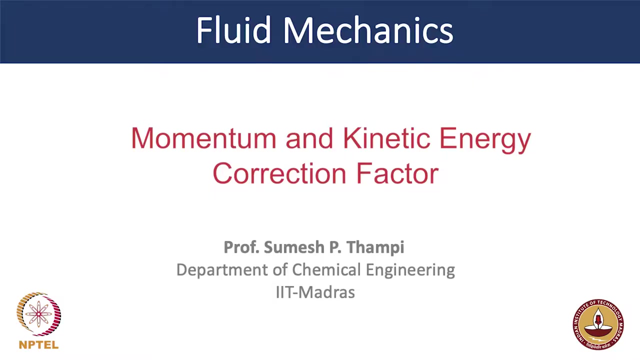 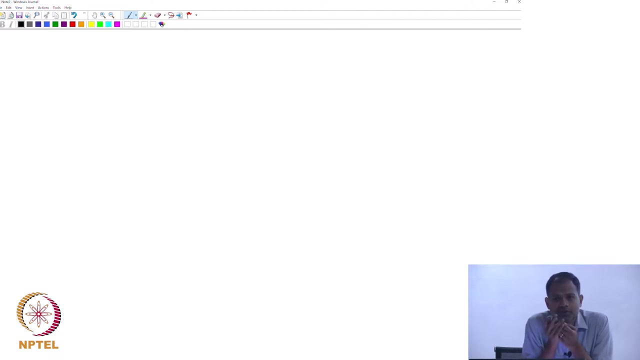 So, I want to introduce you to a two terms that we did not talk about, but you might actually come across these terms and when you are reading let us say books again you are going to see this. One is momentum correction factor and other is a kinetic energy correction. Correction factor ok, these two terms should reallyappear in any of the force balances or energy balances that you write, but I have not been reallytaking that into consideration. So, let me just introduce them to you. So, the first one is momentum correction factor .